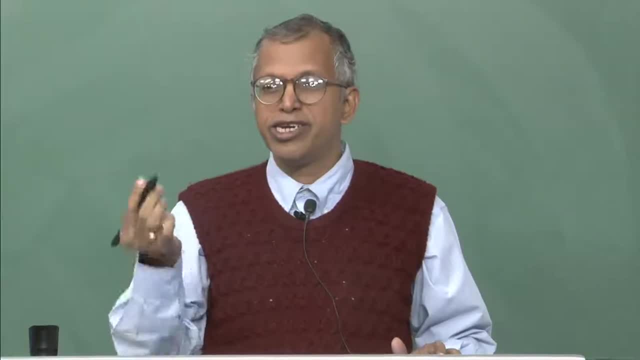 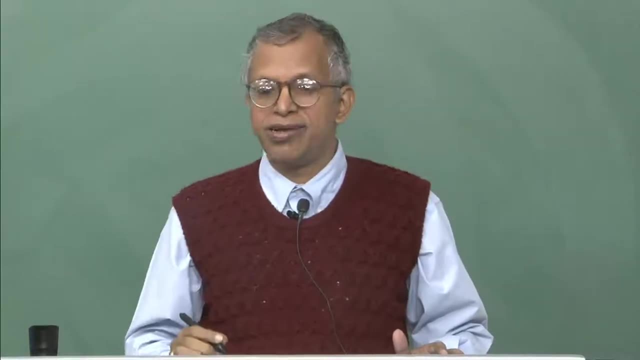 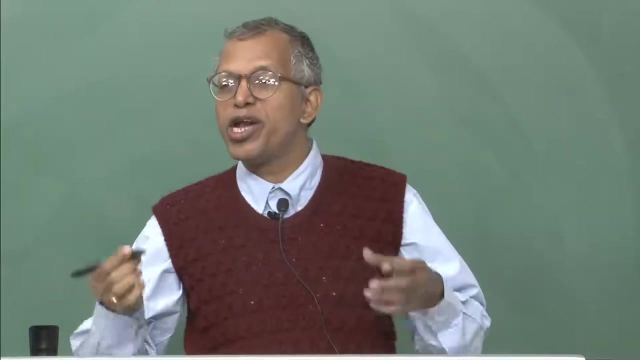 allow the pass due to the gravity you know. like if I take a hole and put it now, we need to disrupt it. basically, atomization is the process of breaking the bulk liquid into the spray or into the number of droplets. right, that means we need to apply certain kind of 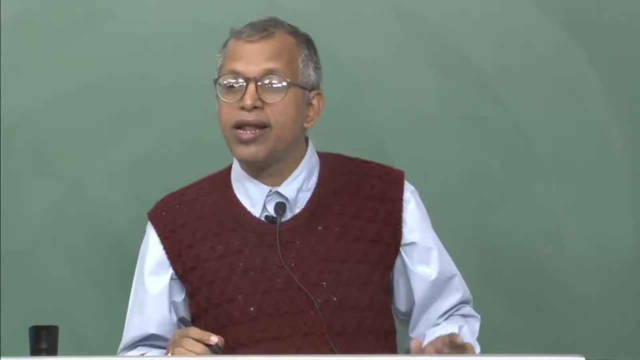 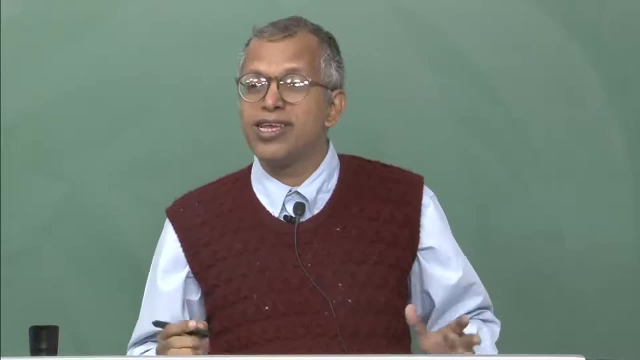 disruptive forces right and that disruptive forces must be greater than what resisting forces right, yes or no? what are the resisting forces which will be acting? yes, in the liquid right? So this is the process of breaking the bulk liquid into the spray or into the number of 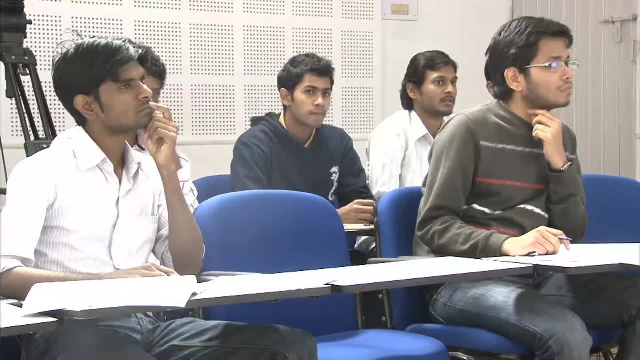 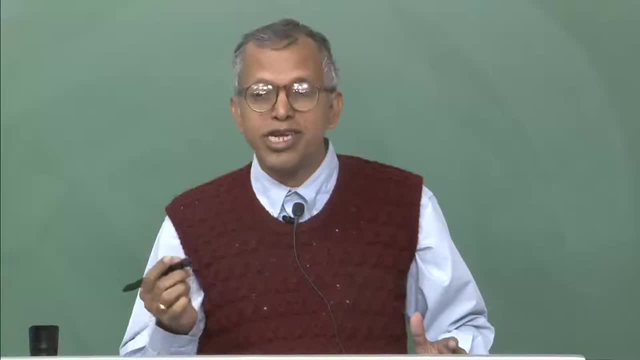 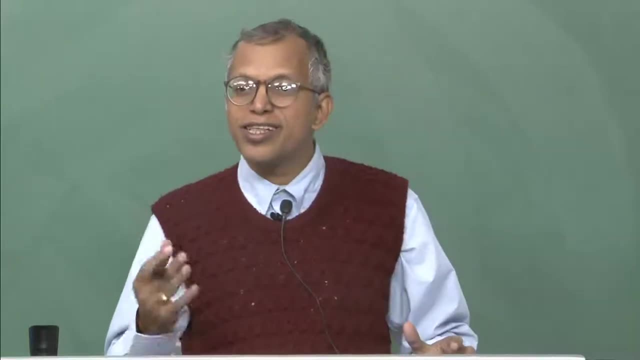 droplets. What are those like? viscosity is one of them, and other is your surface tension right? So whatever you are applying is basically the disruptive forces. what? in this case? it will be gravity if you are not applying the pressure. and if you apply pressure, it will be pressure. 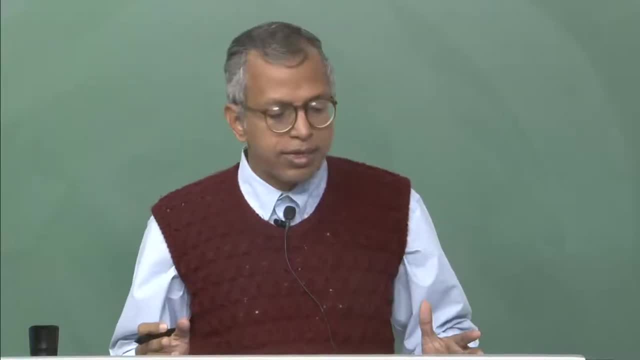 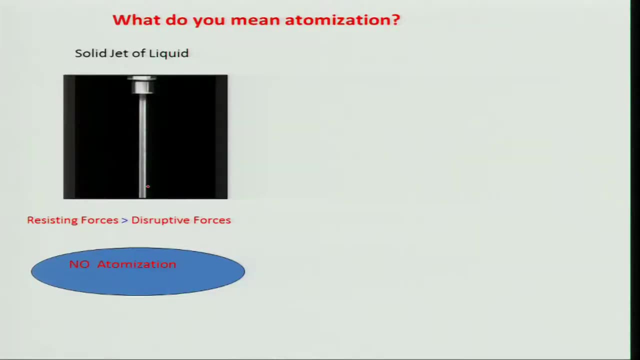 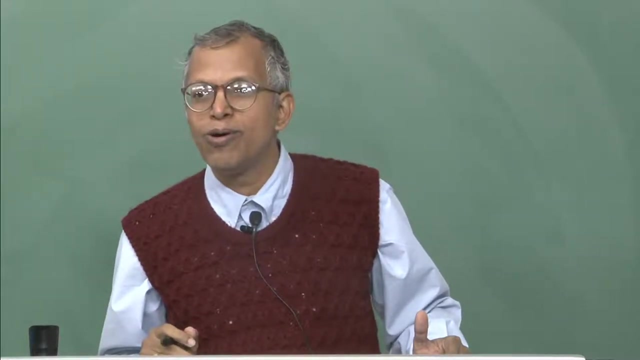 which will be. you know, momentum forces will be acting and other things, and therefore there is no atomization. if you look at right- and that is very important- that means you need to have a higher resistive force than that of the disruptive forces So that you can manage your identity. but if I look at our modern life, what is happening? 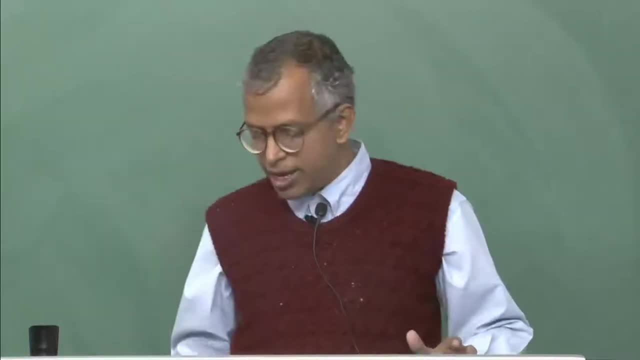 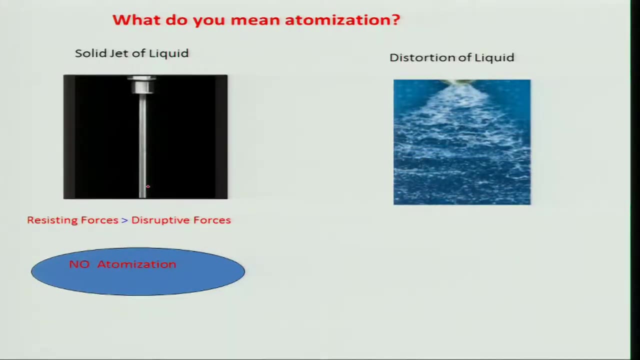 we are getting disrupted, right, we become a kind of thing. So let us look at what is happening to the disrupted liquid. I will go on increasing the pressure right of this, at the upstream of the orifice, which is not shown here. right then what will happen? it will be subjected to instability. of course, 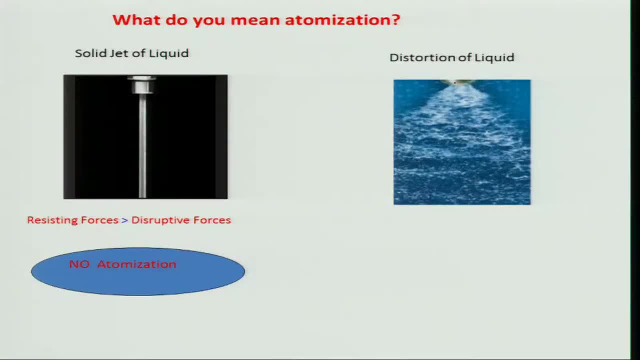 that we called as relay instability and several other. instability is the wavy and the liquid which will be spreading out and it will be interacting with the air and the liquid. if you look at the- So this is the film kind of thing being produced is thin down right. it is a bulk is coming. 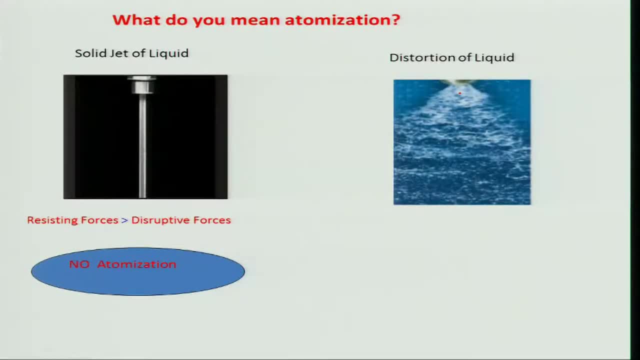 jet. you cannot really break it, So you will have to thin it down. there are several ways of thinning down the thing. right, that means you will be basically disrupting. So what is happening here is that resisting forces is less than the disruptive forces. this is. 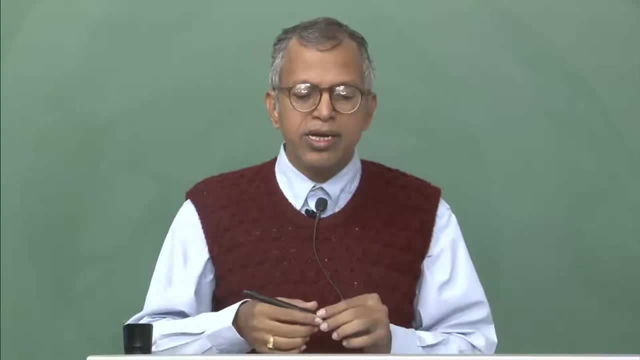 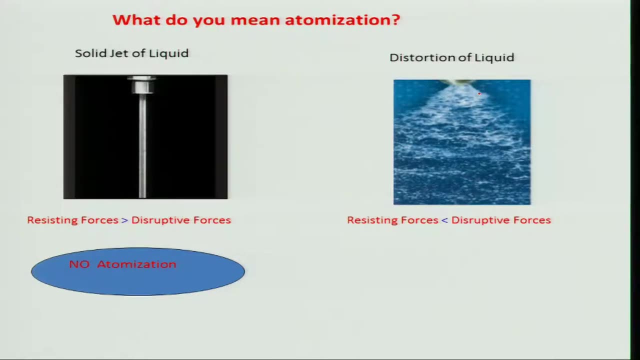 a very simple, fundamental thing right, and then, as a result, this will be, you know, ligaments will be formed from the liquid surfaces And these ligaments will be broken at further and it will be, you know, whenever ligaments and other things from they called primary atomization, then it will be fragmented and 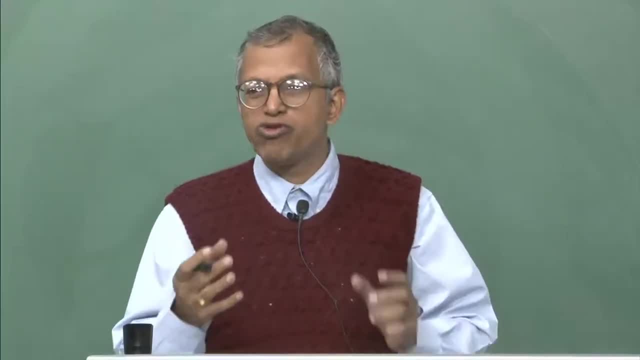 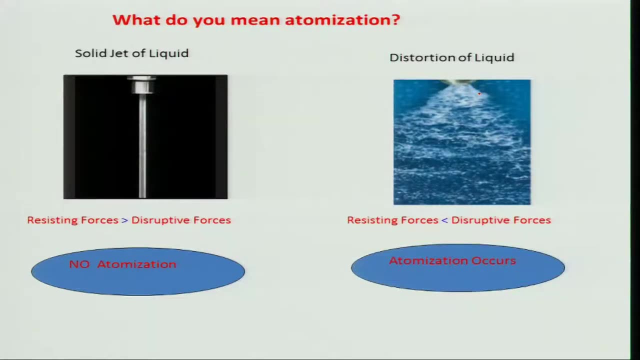 interacting with the air, momentum and other things. together you will get a secondary atomization and droplets. So basic idea is that the atomization occurs only when the resistive forces is less than the disruptive forces. But if you look at our life, our life is that we do not really keep our humanity, we get 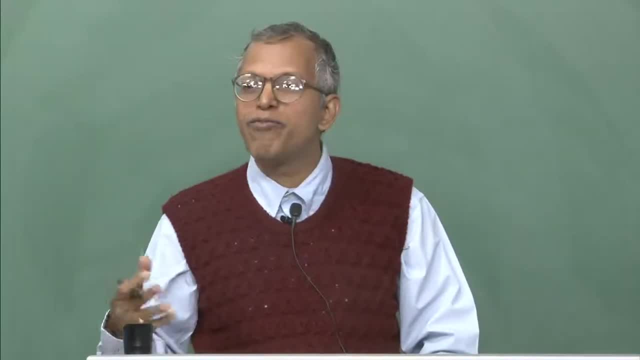 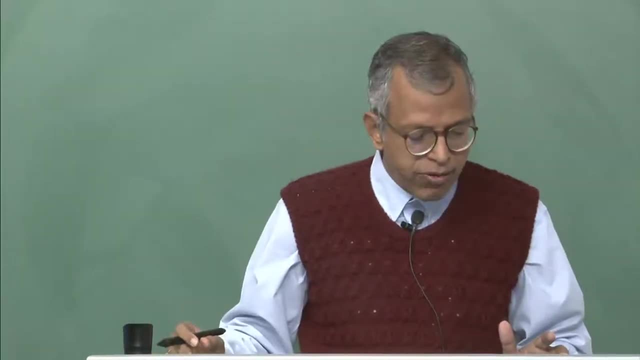 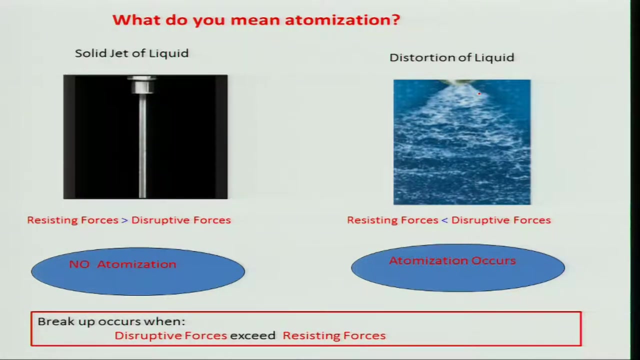 you know, affected by this disruptive forces due to the lack of proper education and control over our forces. So it is a very interesting thing: whenever I look at the spray, I look at the life, you know. Of course, here objective is to look at how to produce the spray, how, 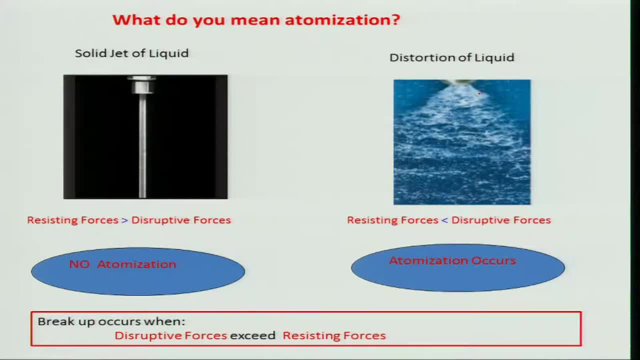 to break the liquid, how to break the bulk liquid into the spray And droplets, and smaller the droplets, better it is for the combustion purposes. So and also it is the distribution is very important. I will be not getting into detail about that. 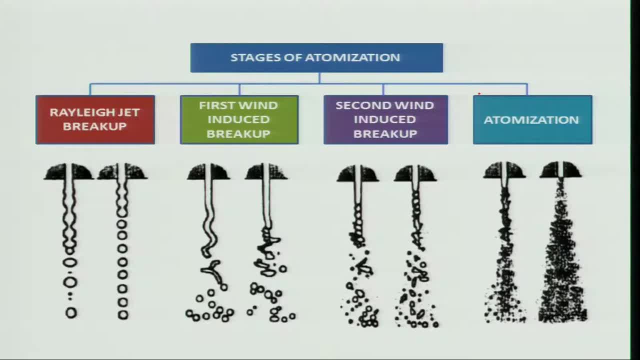 but I will would like to give, tell you what are the stages of atomization. If I take a orifice, if you look at, this is basically orifice, orifice, right, a small hole, and through which the liquid is coming, and if it is coming without really any pressure. So you will find there. 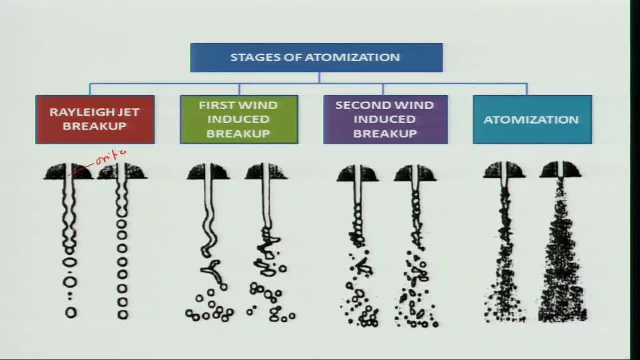 is a undulation. That means it is subjected to kind of a kind of a rallet, jet break of kind of thing because of instability, right, and then there will be satellite droplet and droplet will be coming as you goes on making this little pressure. So you will find this is going up and of 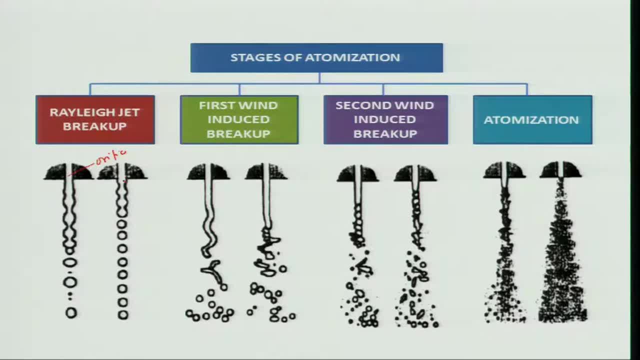 course, there it is not very high, right. And when you apply the pressure more, you know this pressure increases. if you look at pressure is increasing in this direction. in this direction you know injection pressure. So what is happening if the injection pressure? 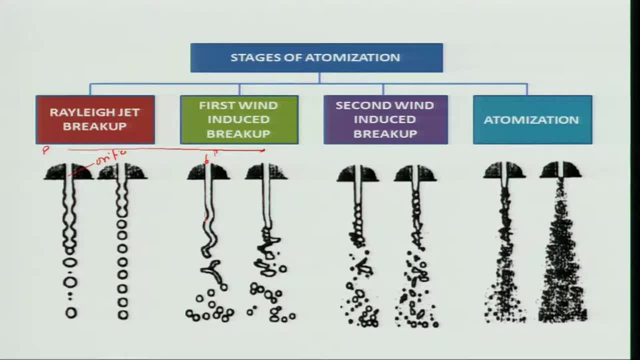 is happening. the liquid become a more stress because the momentum of the liquid is more So. then it become subjected to unstable right and this distance I can call it as a break up distance. you know the length of break up. this is known as break up distance, the where. 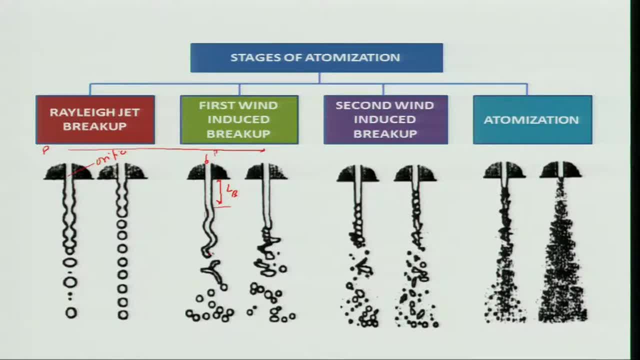 it will be no, actually, basically, if you look at, you can say this is the basically break up distance because this under it is broken out right, this distance and this is the core distance which will remain, you know. So, if you look at, this is l b break up distance. 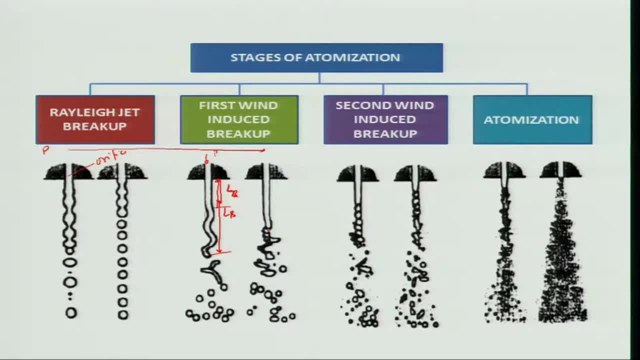 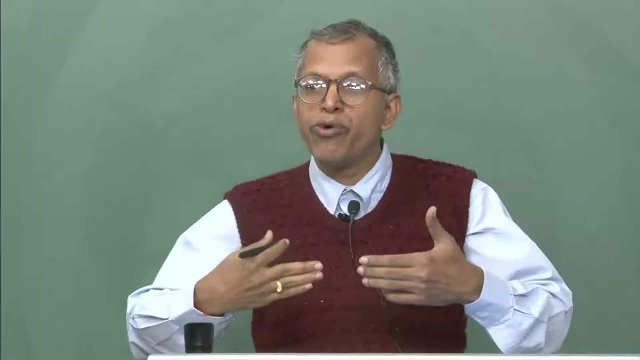 and, as it is you know, pressure increases further. So what happens? this? droplets, you know, like breaks, little higher. that means break up length is decreasing with the increasing in the and in this case the wind, because the momentum is coming, some of the air also will be trying. 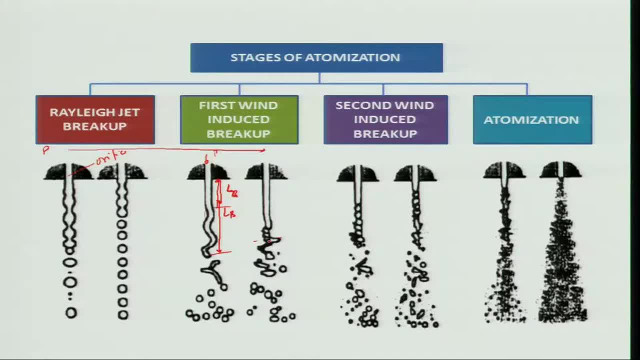 to break up. So this is the break up distance. So this is the break up distance because the momentum is coming to wind and it will be some chipped out, you know, like this kind of thing will be occurring. So that is known as first wind induced break up right and then 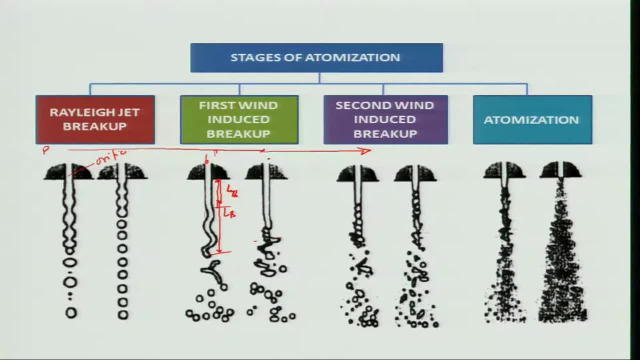 when the pressure increases further. right pressure is increasing along this direction as we are going from left to right towards that pressure. injection pressure is increasing. So then you know, this instability is go above and then oscillation it will more vigorously oscillated So that it will be fluid, will be sticked. 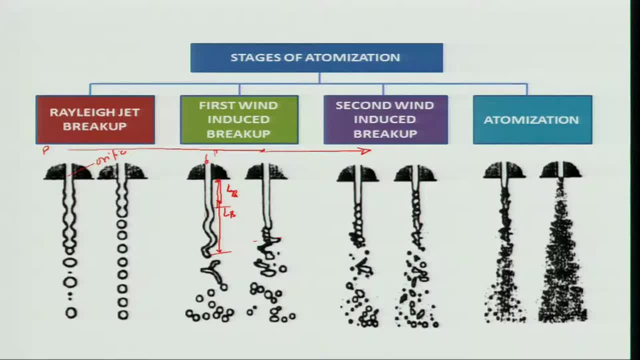 you know, ripped out and then this also goes up and then it is increases further. if you look at, then started breaking of here kind of things. When you to increase further, you know then this is atomizing, is just very nearly to the you know orifice itself. of course, if you look at the angle of this spray also is increasing. 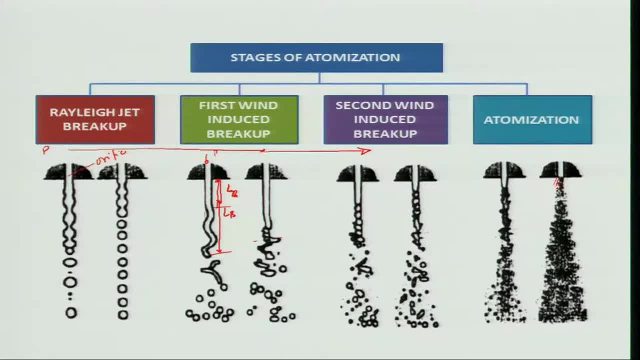 that is also on good thing about that, So which will be helping in mixing kind of thing. So in case of this regime- you know what I am talk was discussing here- the second wind induced break of light means more wind will be coming, entrainment it will be breaking. 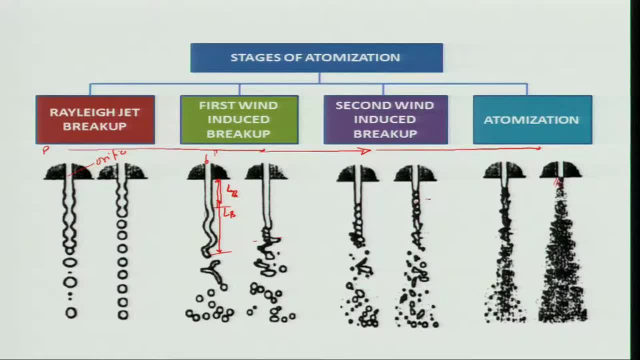 of and the break of distance it goes, you know, becoming reduced as it will go along. So here, of course, the droplet size will be very small when atomization. So we will be operating in this regime of atomization because these are the not being used very much. 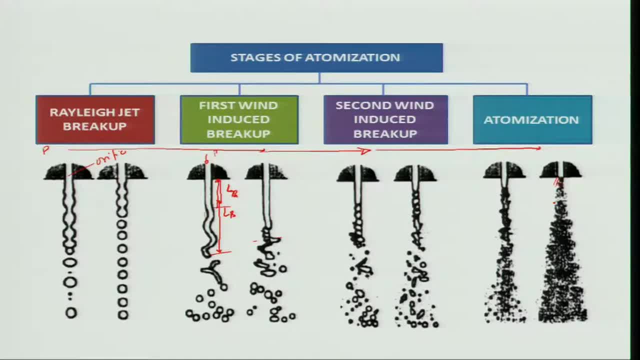 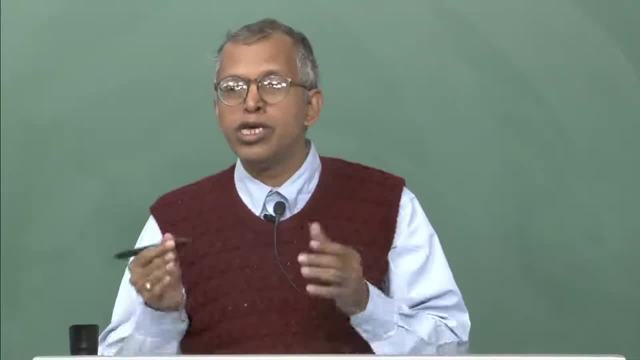 So I would not be getting into the processes, which is quite complex in nature, but what I would conclude? that you need to have a very high pressure and the smaller orifice to have a, you know some meaningful atomization which will be used for the combustion. Now I will. 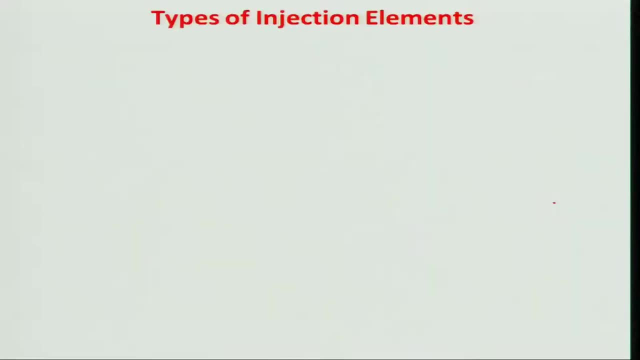 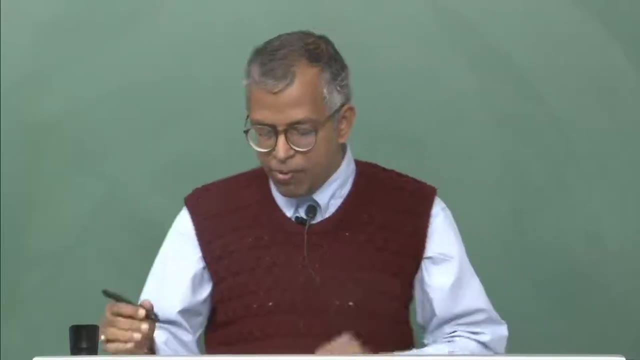 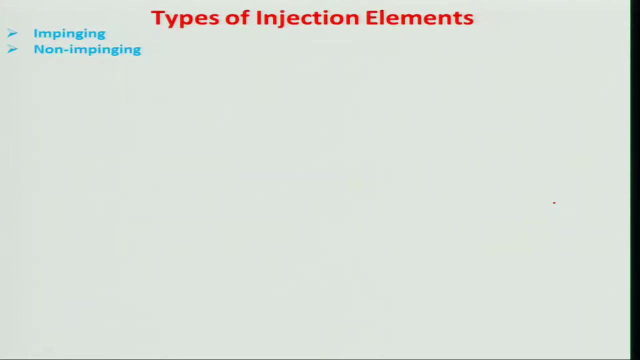 be now talking about. what are the kind of atomizer you know one will be using in a kind of rocket engine, right? So there are. it can be broadly divided in two categories. One is impinging atomizer, other is non impinging- mostly the impinging atomizer being used in 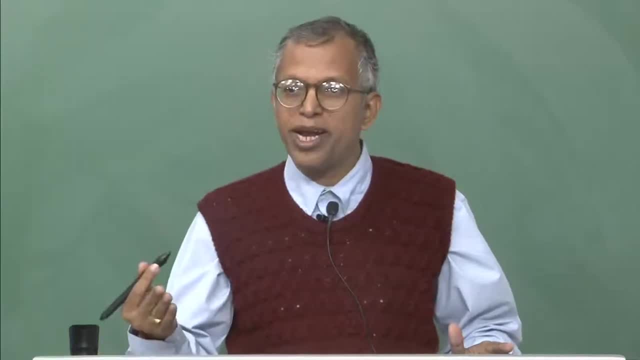 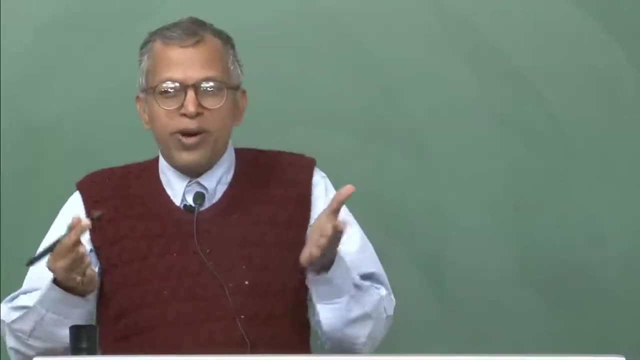 case of which? propellant? liquid propellant definitely, but non impinging also, we will be using for non liquid propellant. Whenever atomization is concerned, it is about liquid. we would not be atomizing the gas, nor atomizing the solid, so naturally it will be liquid. 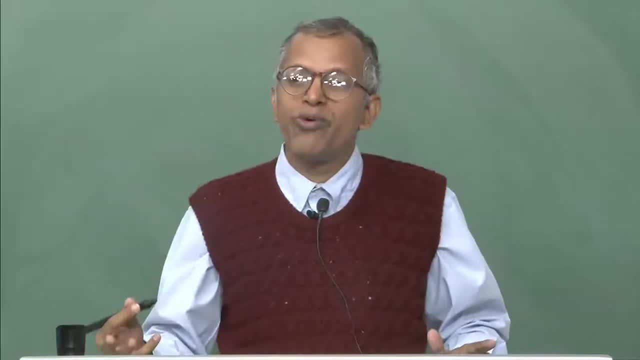 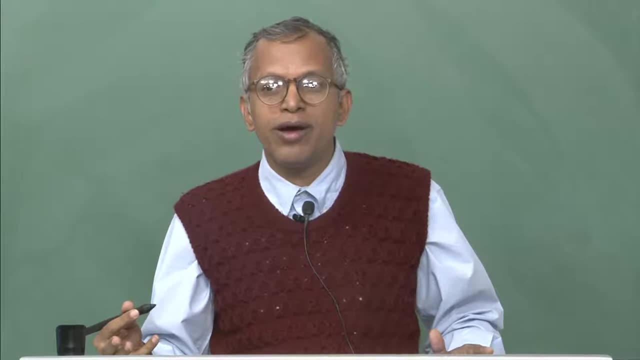 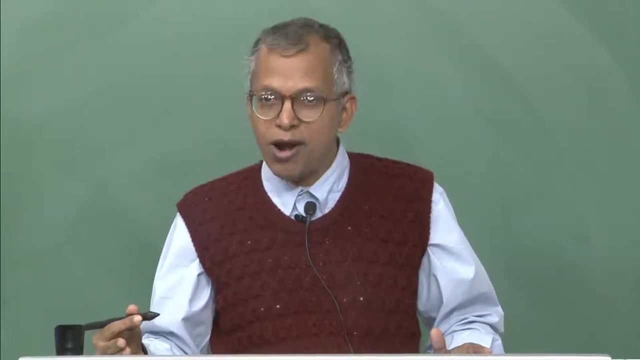 but what kind of propellant? 5.37. there is two propellant we discuss about. one is hypergolic, other is non-hypergolic. So in case of you know, in impinging one, what we will be using, We will be using the hypergolic. 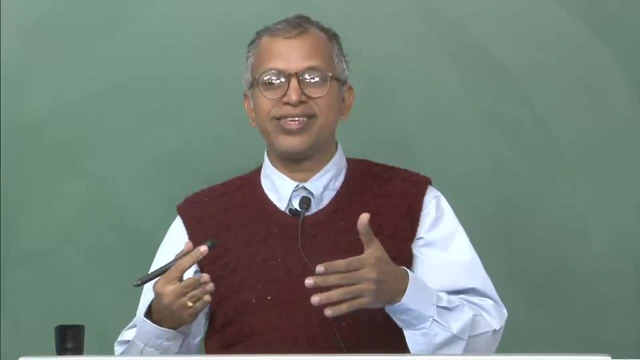 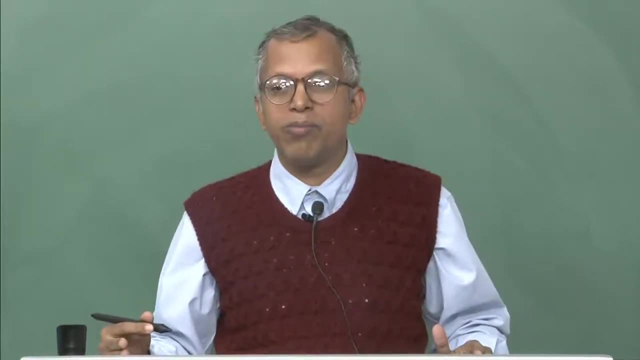 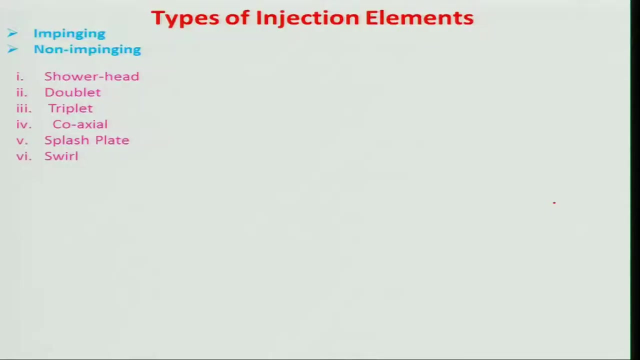 not non-hypergolic, because we need to mix this by propellant. of course the propellant can be by propellant, monopropellant, But particularly when we are talking about the by propellant, we should have the impinging, but not all the time. as you go along, we will. I will discuss. 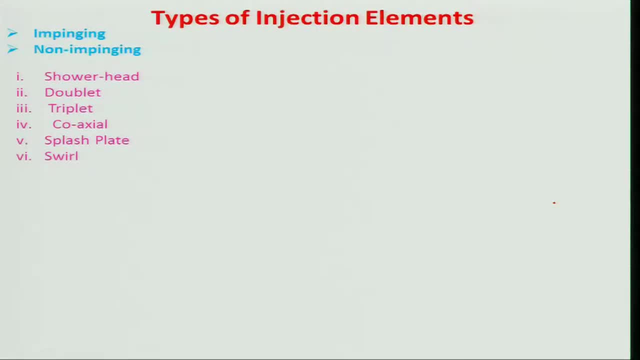 about this. So some of the injectors I which I will be discussing is shower head, doublet, triplet, coaxial plus plate and swill, but there might be several other varieties which being developed and design, because that depends upon the requirement and also the creativity. 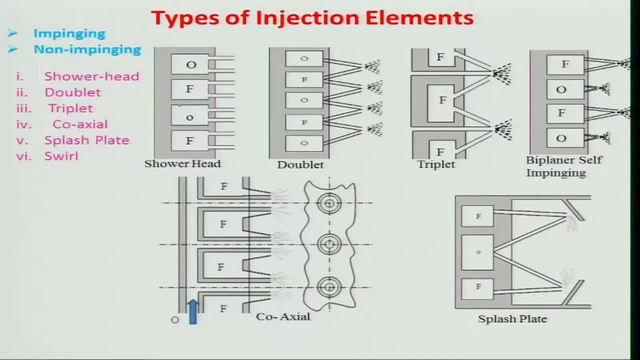 of the person who is developed. So that is very important. So, if you look at, this is the first one. So what we are looking at here is the shower head. shower head means it will be having a straight orifice right, which is like our shower, what we take the bath in every day. 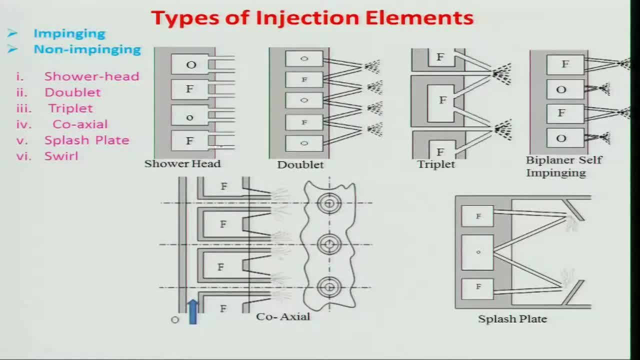 it will be going straight and, of course, this is a fuel inject. this is for fuel and this is for oxidizer. As a result, what will happen? it will be converting into spray, depending on the pressure, but it will take more time for mixing. as a result, the length of the combustor. 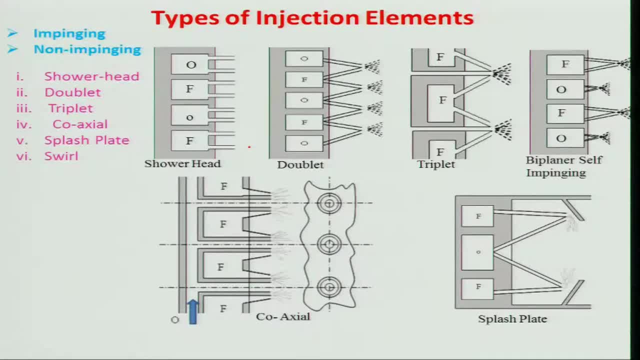 in this case. So it will be higher. but the one advantage is that length of the combustor may be higher but the heterogeneity of this fuel and air will be more in the near the injector head. like, if you look at, this is your injector head right, So the flame or the combustion 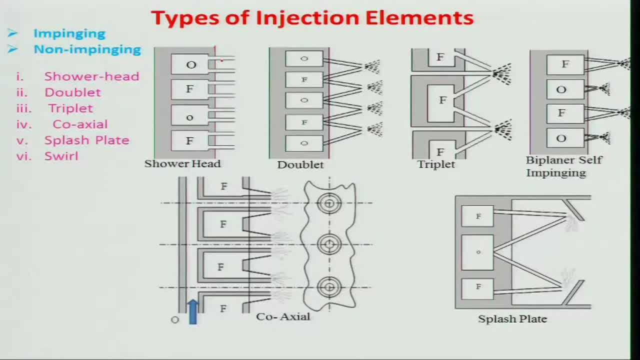 will be taking place little away from the your injector head. So this is your injectors head, right. So thus the, you know the temperature or the heat cannot really be affected by the combustion. So it will not really come, not much. you know will be coming towards the this. 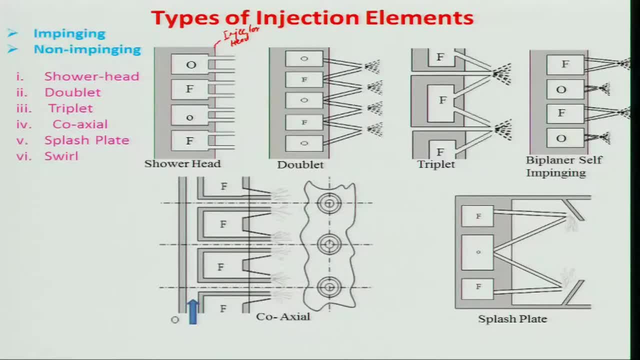 injector head and you know the fuel properties would not be getting affected because you know, like fuel property and there might be also a carbon formations and other things would not be there, which is very important for the clogging of the atomizer, for the performance of the atomizer. So, but however, you will have to pay a penalty the length of the combustor. 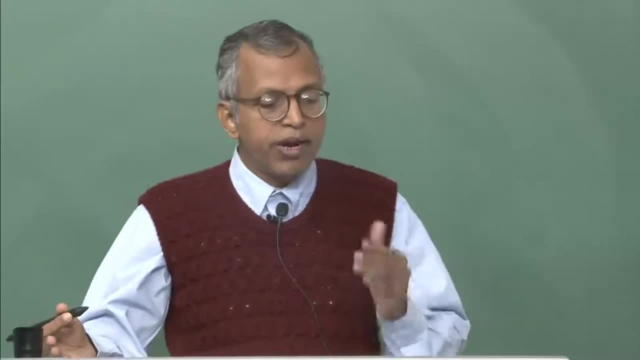 will be high, then it will become heavy, and then you know all those things. but if you look at this, shower head is being used in earlier rocket. So that is what we are looking at here. So that is what we are looking at here. So, 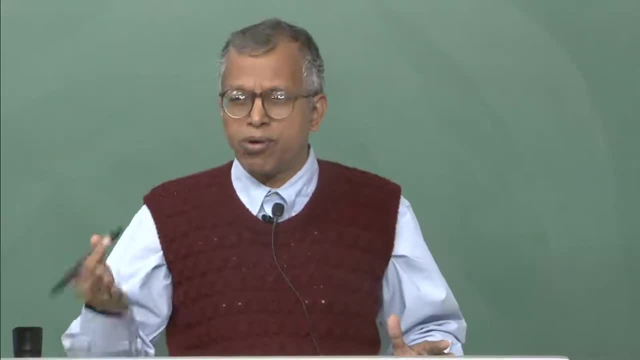 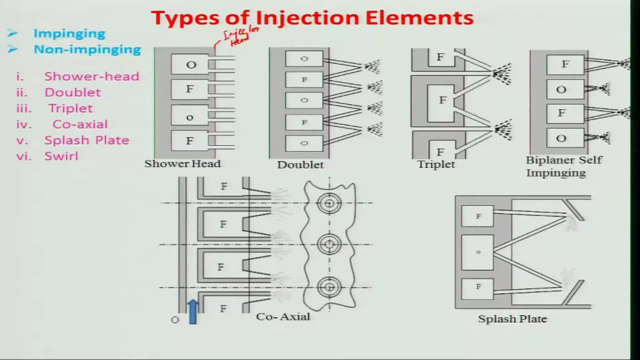 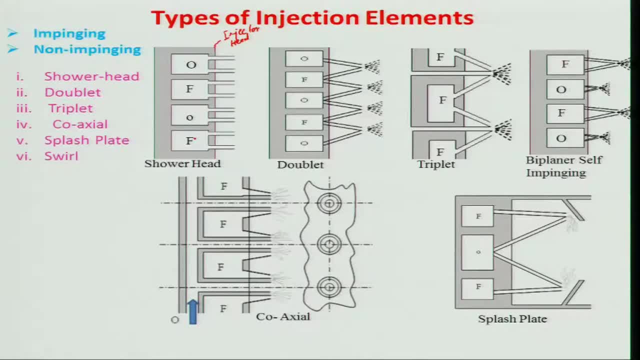 also the shower head can be used for the non-hyperowling you know. prop them where you need not to mix fuel and oxidizer to have a liquid phase reaction, But where has, in the hyperawling, we need that fuel and oxidizer to be mixed, which will be spinach. So it is also- you know this- chemical. 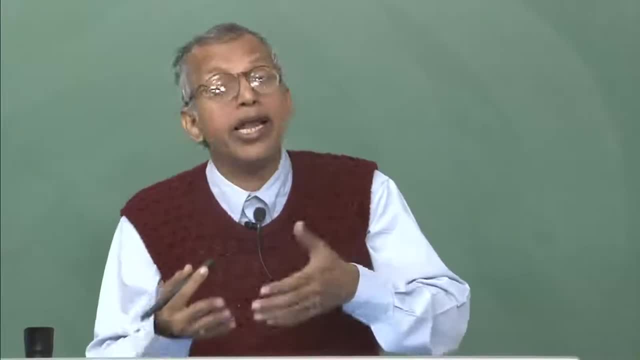 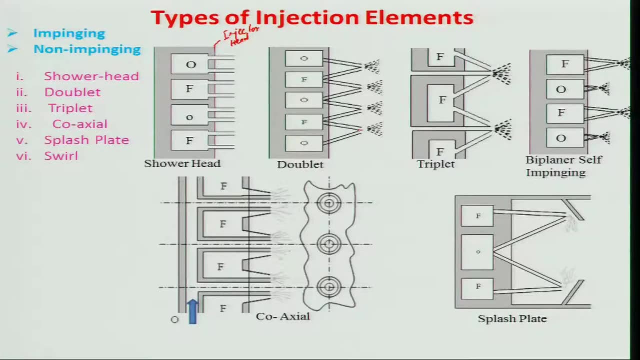 what is the answer? this is what is initiate problem, where you need to study this going liquid phase So that some heat can be developed and it can ignite itself. So, therefore, doublet is being used and it is a one good part is that it is being mixed at the, you know, at. 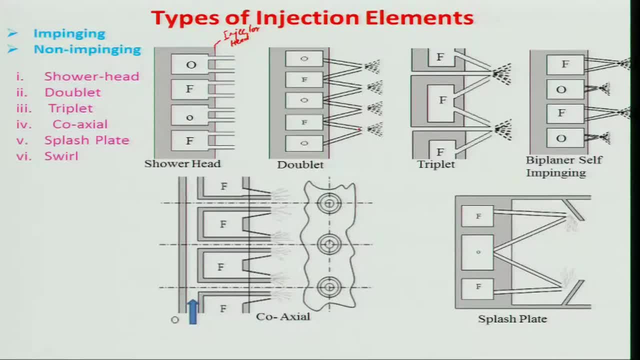 a particular point, whenever it will be impinging on each other. there will be a in this zone, there will be a fan which is being formed, and then fan will be formed perpendicular to the what you call the plane which I have drawn here, and this fan will be interacting. 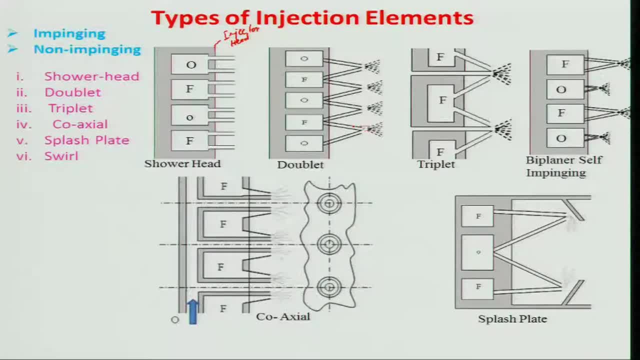 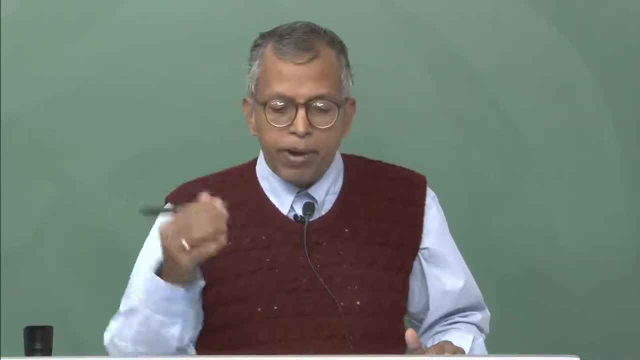 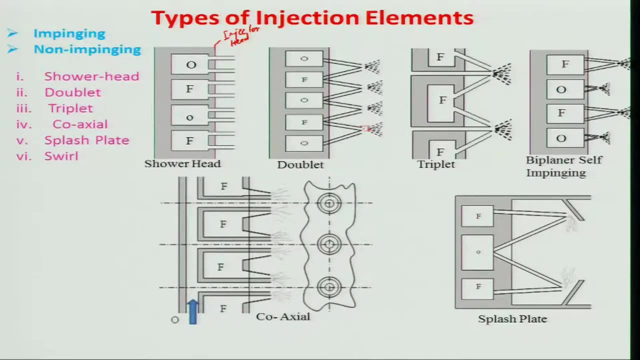 and you know, with the air, and then it will be also chipped out those ligaments and then form. But problem is that this kind of course, that the droplet, the size of the ligaments which will be formed, will be dependent on the thickness of this fan which is formed and it will be subjected to instability as well. The problem: 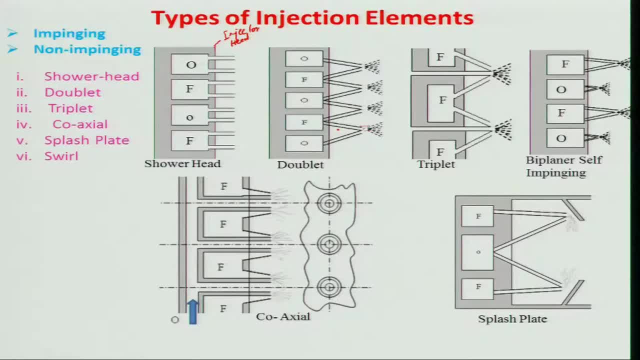 with this. suppose you know, like we know, that we need to have a higher amount of heat and we need to have a higher amount of oxidizer as compared to the fuel. So therefore, for the same size, or if it is, then the momentum will be higher for the oxidizer as compared. 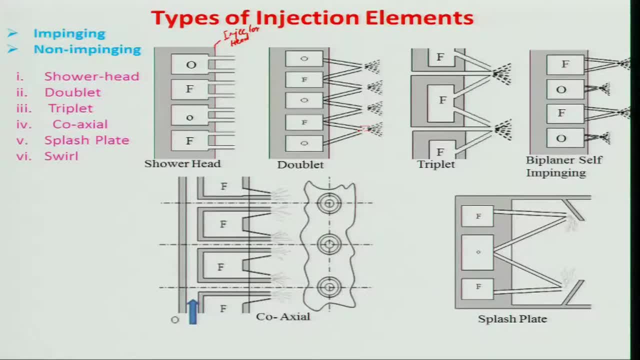 to the fuel and sometimes we will be using. of course one can design such as that momentum will be similar. But if it is one of the momentum of the oxidizer or the fuel is higher, then the meeting point will be different, meeting impinging point will be different. and if that 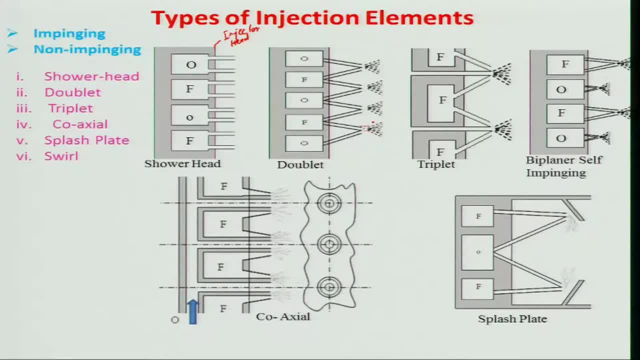 is different, then naturally, your performance will be very different. So that is the problem. So, in order to overcome that problem, what is being used is the triplet, where you will have the oxidizer. you know it will be coming in the center and there is a fuel, and then 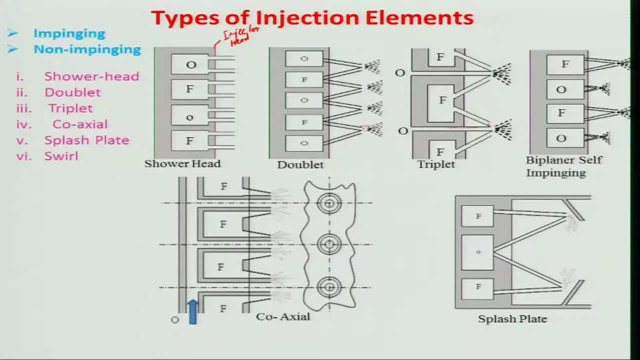 of course the fuel will be coming over here and then this is can be again used for the hypergolic propellant. But you know, it does not matter if one of the you know this thing is being higher and oxidizer being higher. it will go little away, but you can manage. 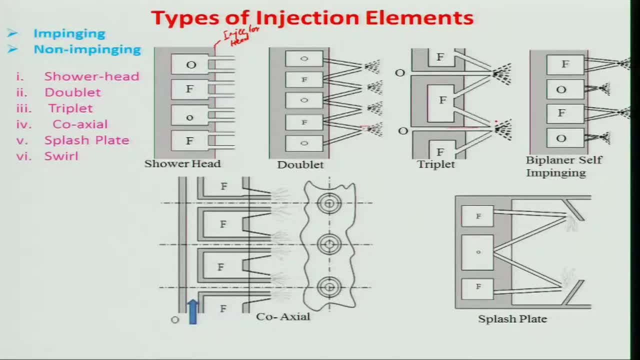 to have that. But even. but if there is a very, very high pressure, then it will be leading to the problem. But you know, there is the liquid phase. combustion will be taking place, liquid phase reaction will be taking place and also it will be compact. 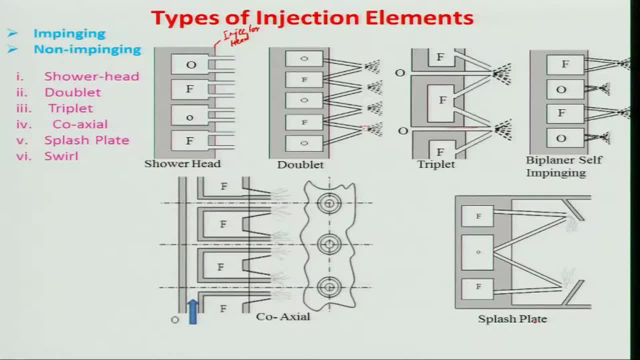 and nearby. But if you face this problem, there is another one which we can think of using is known as a splash plate. So use the doublet right. this is basically doublet kind of thing, But however, there is a flash plate in case of this impinging point. not here it will go. 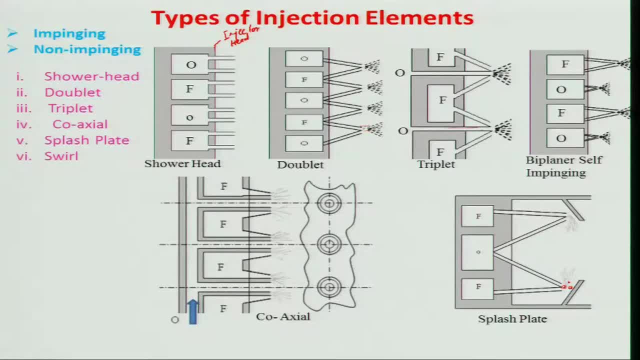 to here. it will impinge into the Video Lecture on Experimental Stress Analysis, Prof K Ramesh, IIT Madras plate itself and then, so that you know, you can convert it into ligaments and will do that. but there is a problem because if it is hyperglyph and this will be heated and 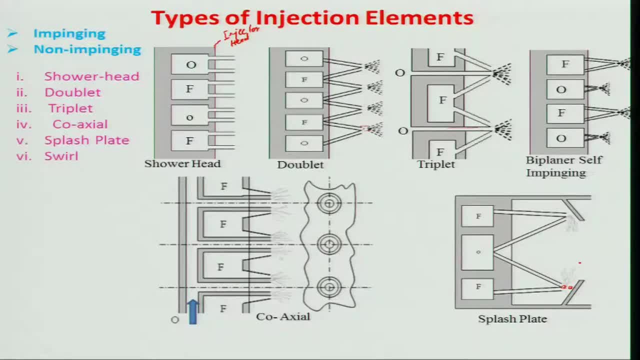 then you know you are having to pay some penalty for that. So there are several varieties. if you look at this is known as the unlike impingement that fuel and oxidizer like and in. sometimes we use for the like impingement, like oxidizer. 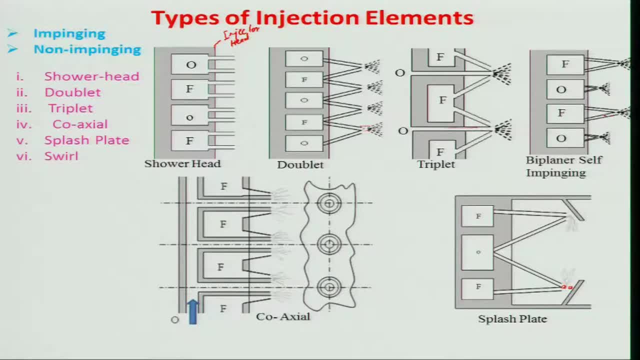 that is impinging into oxidizer and fuel is impinging into fuel, in this case biplaner, self impinging- you can call it as self impinging atomizer kind of thing. This generally is being used for the non-hypergolic propellant right where it is not required to ignite you. 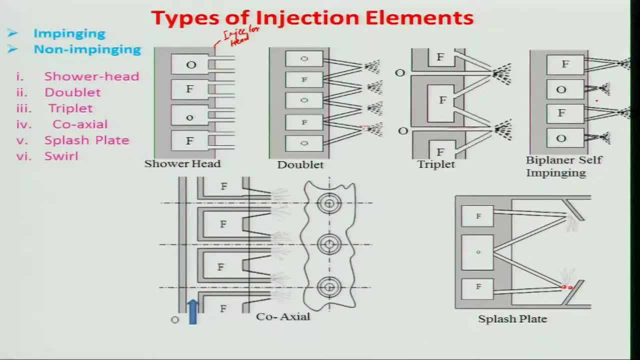 need to have ignite separately. there is no need. I mean, there would not be any liquid phase reactions which will be occurring. So therefore it will be. but, however, here your mixing time should be more, So that it will mix. oxidizer will be mixed. 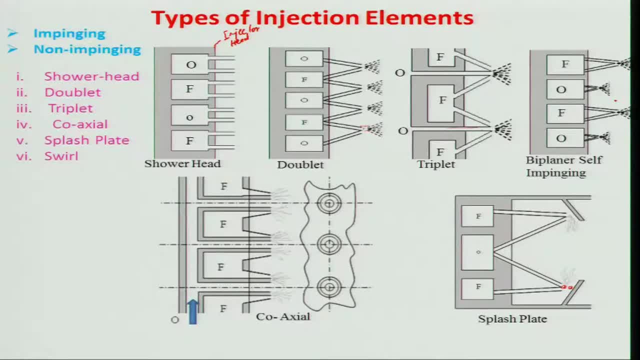 with the fuel and gas phase. then may be liquid, you know droplet, and then you know vaporization, all those things. So length of the combustor in this case will be higher. So that is the you know like, but it is used for the non-hypergolic propellant. 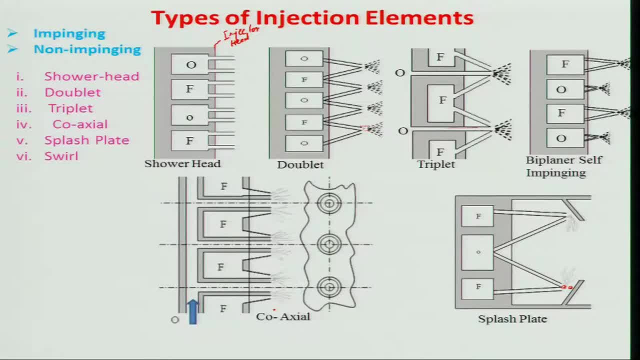 There is another one which is used very much, particularly for the cryogenic engine. that is known as coaxial kind of atomizer. If you look at, the oxidizer is going through here and here and in this case, and it is having the fuel. So that is the one which is used for the non-hypergolic propellant. So that is the 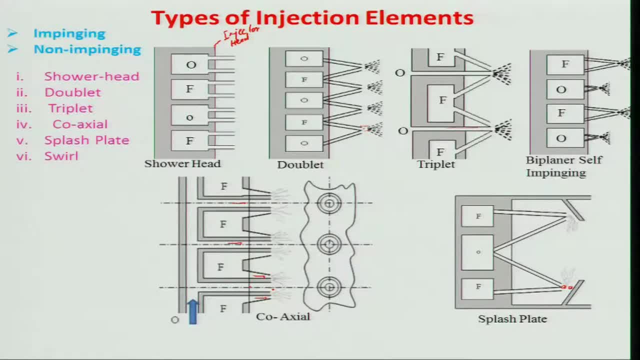 fuel is, you know, passing through this and it is a coaxial in nature, So that what will happen, like if you look at in this case, that cryogenic engines or the any other liquid, the fuel is being used as a coolant to cool the conversion diversion nozzle and also the 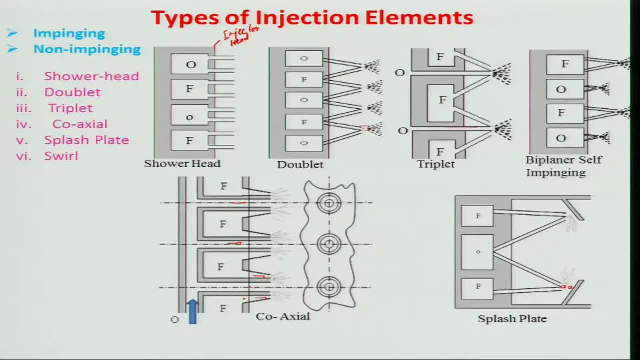 body and heat carries, and mostly it will be particularly for liquid hydrogen. it will be very high, So it will be the capacity which will be coming. it will be very high. it will be order of may be 300 meter per second, whereas the liquid will be passing through the kind. 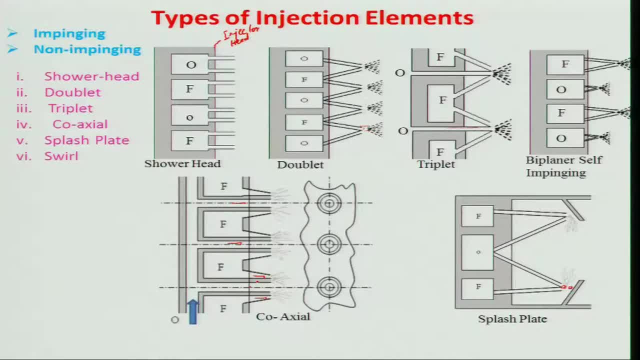 of what you call very low velocity order of may be 30- 40 meters per second. So therefore, this will be basically gas momentum, which is a lighter one, which will be because you need to have higher moment to interact with this, and then do that In order to augment. 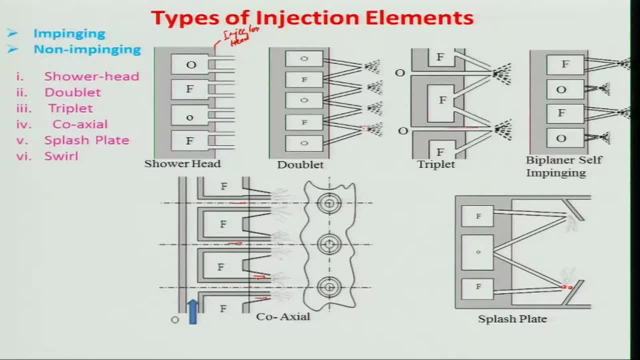 the performance of atomizer. people recesses. That means what they will be doing. they will be, you know, not in the same plane of the atomizer, both the what you call oxidizer and the fuel. they will. instead of this, they will start here. you know, like there will be some zone. 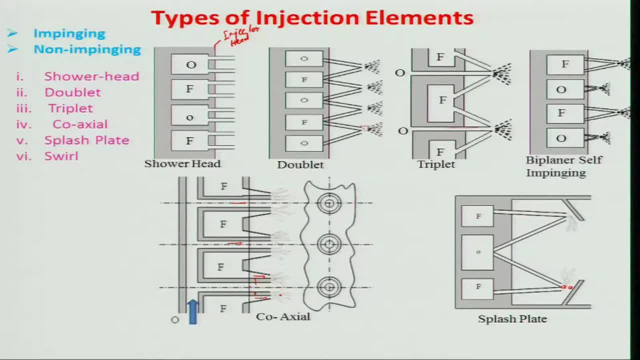 where some mixing will be taking place between the liquid and the oxidizer, the liquid oxidizer and the gaseous fuel, So that it will be two phase flow and then you will. so that is basically is known as internal mix atomizer people are using now 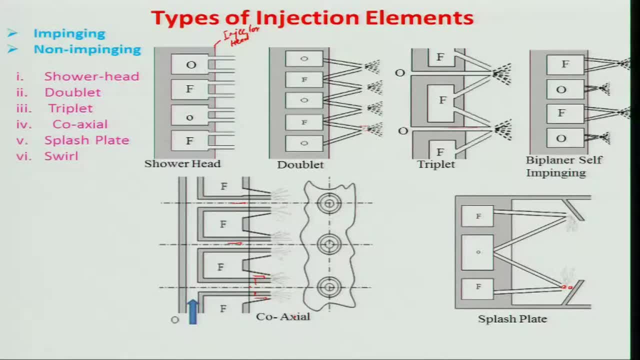 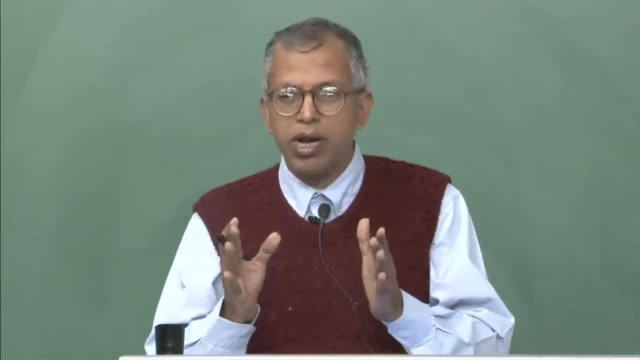 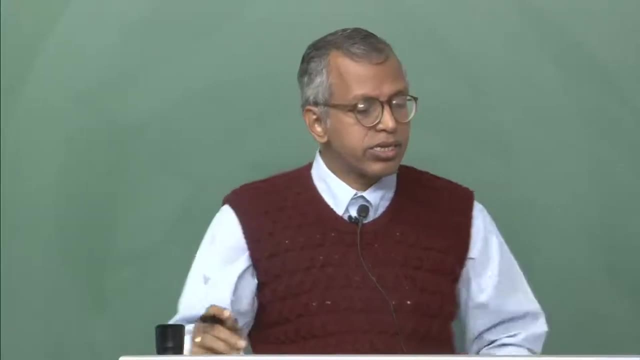 a days. this is a modern design and in order to overcome, you know, this problem of mixing and then good atomization kind of thing and compactness of the what you call the combustors, people are thinking of using a swill that means they will pass this, you know, as basically. 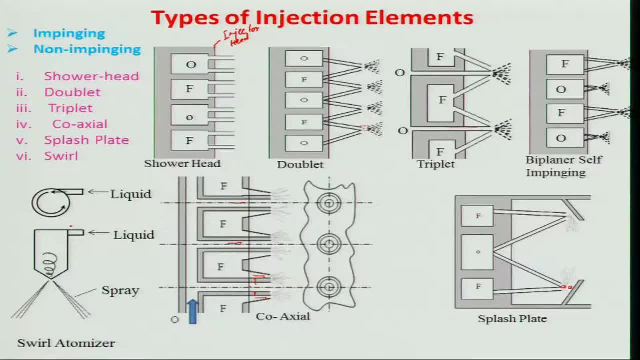 a liquid which will be passing through a swiller, the tangential entry, and then it will be having some angle, it will be fixed And the you know, the liquid film will be thin down when it is centrifugal force being acted upon. that and then, from this, here you. 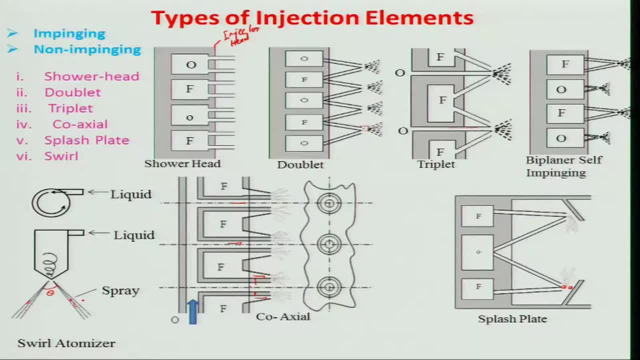 know, liquid will be coming out and then droplets will be, ligaments will be formed and will come, So that what happen it is going towards that and then mixing will be better. of course it will be having a, you know, a hollow cone kind of thing. sometimes will be solid cone. 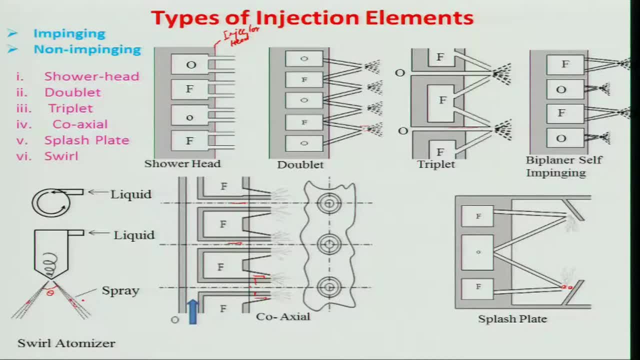 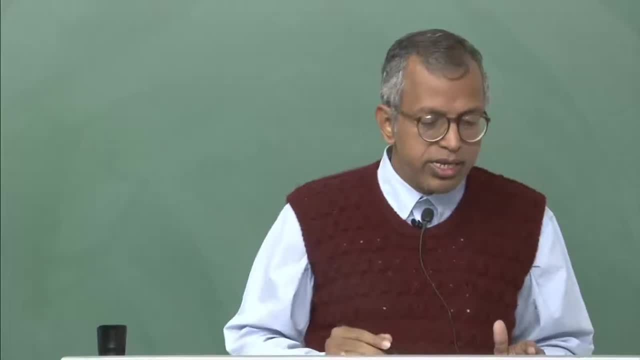 as well. right, But what is important? that it should be hollow. but the distribution of the atomizers or the droplet also little bad. Video Lecture on Experimental Stress Analysis by Prof R Ramesh, IIT Madras. So you need to look at it. it is generally the swill being used, even in the coaxial kind. 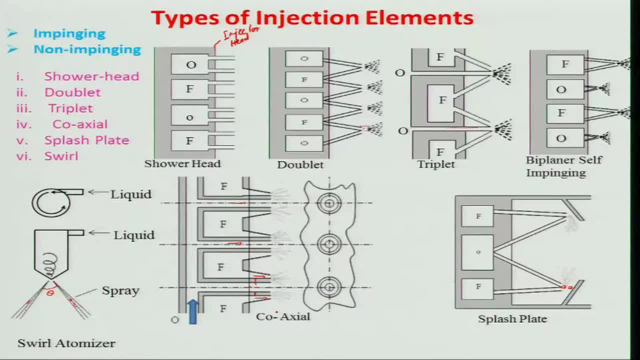 of thing right. you can make it swill as a fuel, particularly in the oxidizer. it is being used and sometimes it is being combined with- you know, fuel also. So there are various varieties and various tools. these are, if you look at, is the elements or ideas are available. 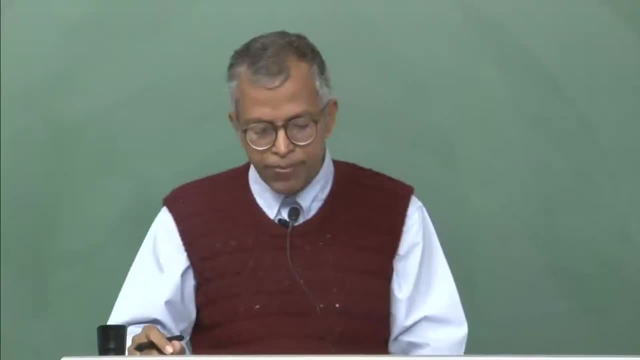 one can use it for different applications and other things. So generally this coaxial kind of thing is being used. Video Lecture on Experimental Stress Analysis by Prof R Ramesh, IIT Madras. So generally this coaxial kind of thing is being used for the non hypergolic propellant. 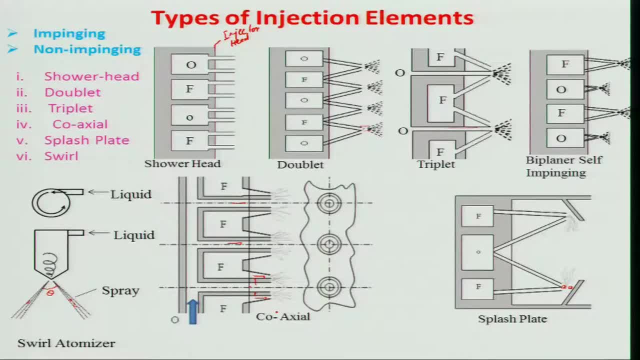 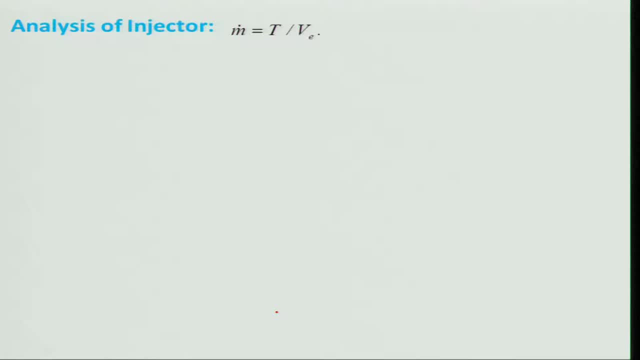 and impingement generally being used for the hypergolic propellant right. So let us look at some analysis of the atomizer. I will just look at quickly. we know this thrust expression. the mass flow rate of propellant can be, you know, express in terms of thrust and exit velocity. 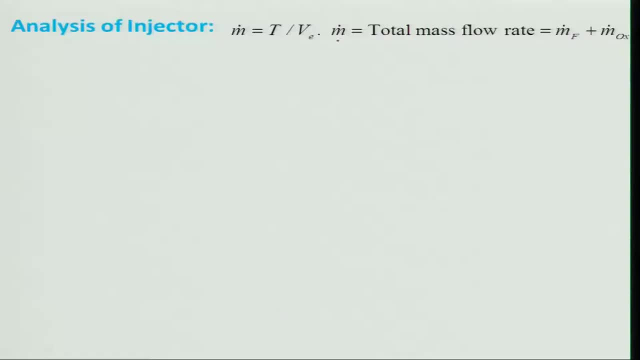 or equivalent velocity you can use. So what is the total mass flow rate of the this thing? that is nothing. Video Lecture on Experimental Stress Analysis by Prof R Ramesh, IIT Madras. The mass flow rate of fuel and mass flow rate of oxidizer. suppose what I will do. I will. 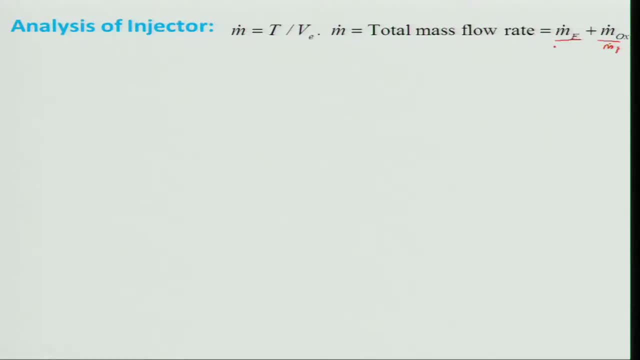 divide this by the mass flow rate of fuel, right, and then it will be cancel it out, right? if I say this is oxidizer flow rate, you know, by the mass flow rate of fuel is known as mass ratio, right? m r, that is the mass ratio. then I can get an expression: m dot f is nothing. 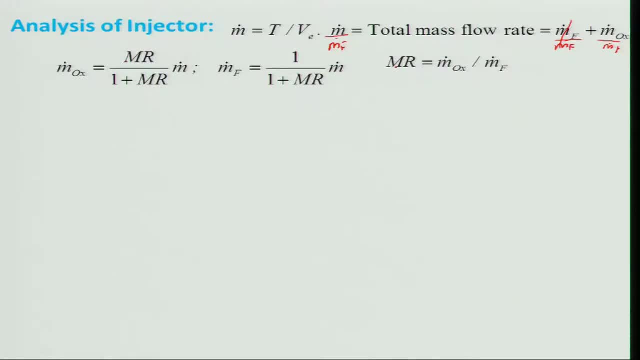 but 1 over 1 plus m r. Video Lecture on Experimental Stress Analysis by Prof R Ramesh, IIT Madras. That is the mass ratio into total mass flow rate and similarly I can get an expression for the mass flow rate of oxidizer in terms of mass ratio and mass. total mass flow rate. 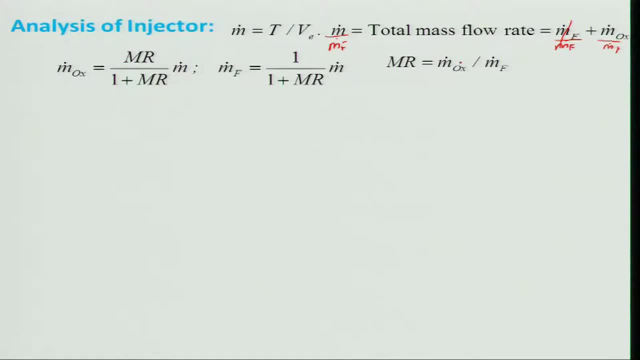 keep in mind that you should keep this in mind. that is the ratio. mass ratio is basically mass flow rate of oxidizer divide by mass flow rate of fuel. in some places people do other where you will have to be careful, So by what we will do. if I take an atomizer, 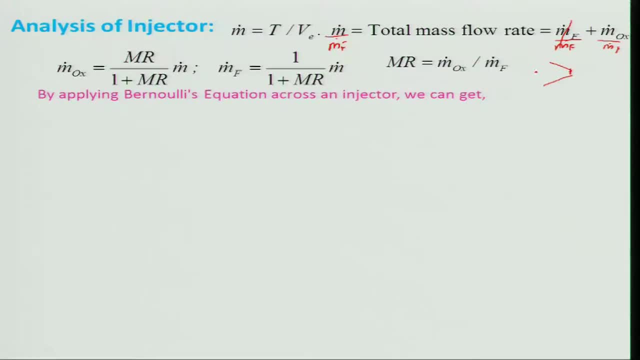 kind of things. you know, this is a small hole here and the p c is being applied here, and this is having certain velocity, v, right, it is a orifice, orifice through which the liquid is being pressurized. you know, right, I can apply a Bernoulli's equation. of course, the 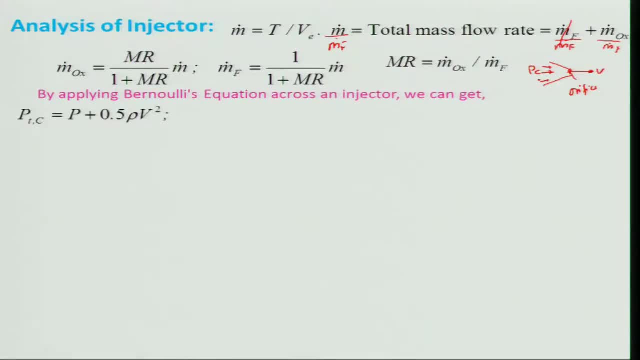 losses will take care by differently. and that is p. t c is nothing but your local that is. p is the static velocity plus half rho. Video Lecture on Experimental Stress Analysis by Prof R Ramesh, IIT Madras V, square v is the velocity at the nozzle or the orifice. So if I look at, I mean then 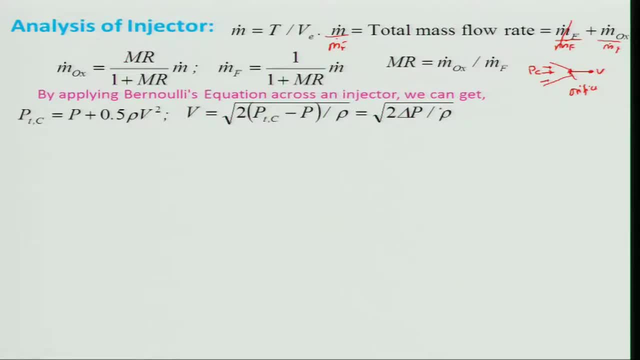 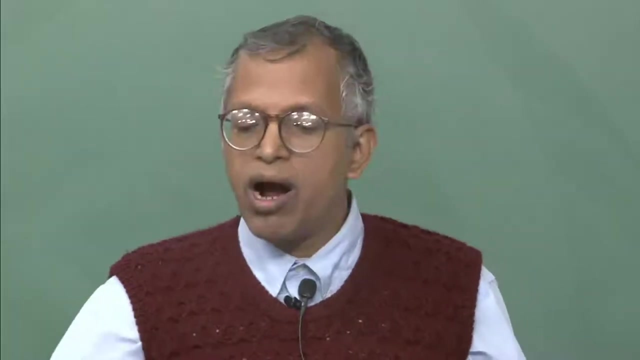 velocity will be basically root over the change in pressure divided by the density, density of the liquid right, So for, but that is for the ideal, you know, in which there is no losses, no separation, other things So. but whereas in real processes there will be contraction. 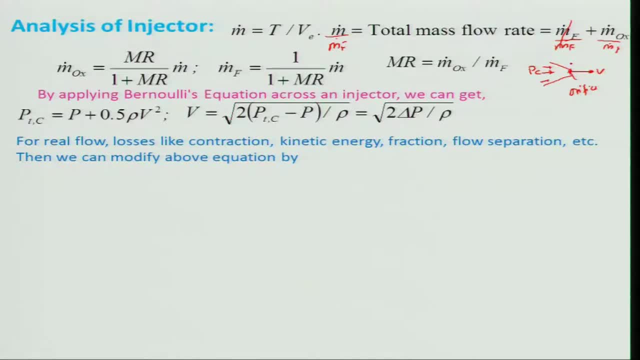 like this. it has to be contracted and there is a flow, separation may occur. there is a friction right and it can be. we can modify this equation by using a quantity. we call it c, d. c. d is basically viscous coefficient and that is the actual, you know, flow rate. 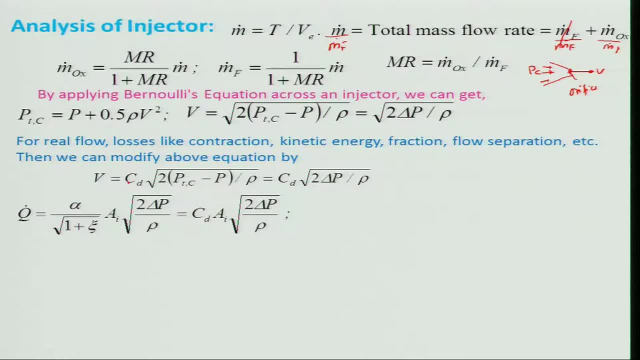 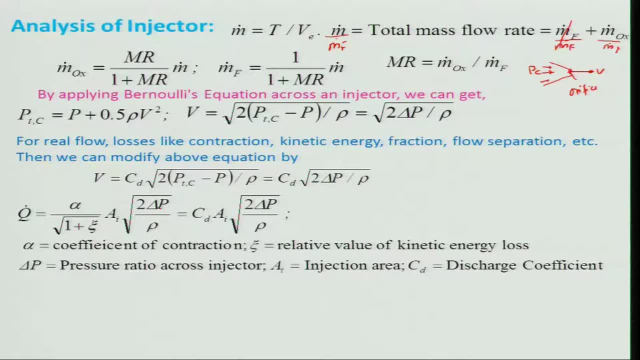 1 plus 1.5 into a plus 1.5 into a plus 1.5 and put that as theta into a I and root over two delta p by rho, then if you look at, alpha is a coefficient of contraction. that means how much it is been contraction. what is area ratio between this inlet? if I take this inlet, 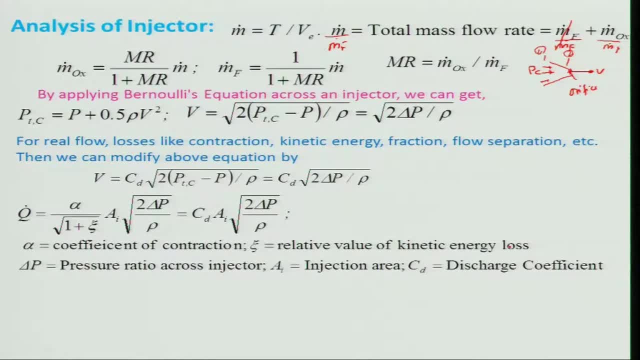 and if I take this outlet And relative value of kinetic energy loss, that energy loss will be there and delta p is the pressure ratio across the injector and a- i is an injected area, cross sectional area at the- you know- exit of this orifices. 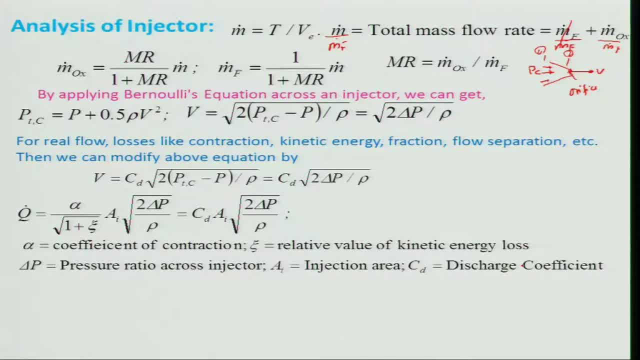 Let me tell you now this: we have already done phase two phase. I have already tried the phase one, phase two, phase one, phase two phase. I have already body phase period where there is Douglas and C, D is the discharge coefficient. So what I will put all these together, you know. 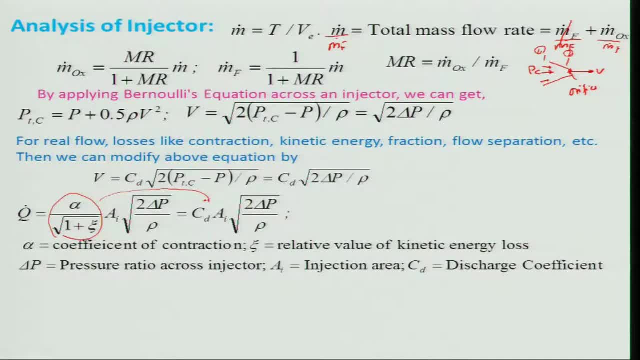 I can put into as a C D, like you know for a, because when I am conducting I need not worry about that. I will just put into C D. And if I express this in terms of mass, you know mass flow rate, that is nothing but rho into volumetric flow rate. this is q dot right. 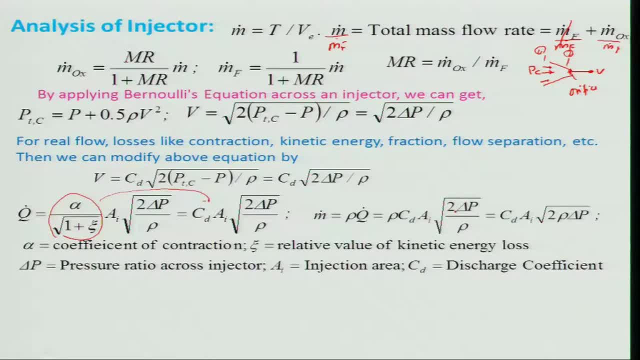 into rho, into C D a. I can get C D. if I just take inside, I will get C D a. i root over 2 rho, delta p. rho is the liquid density right, delta p is the pressure across the orifice or the injector, whatever you call it, basically across the injector. that is the right one. 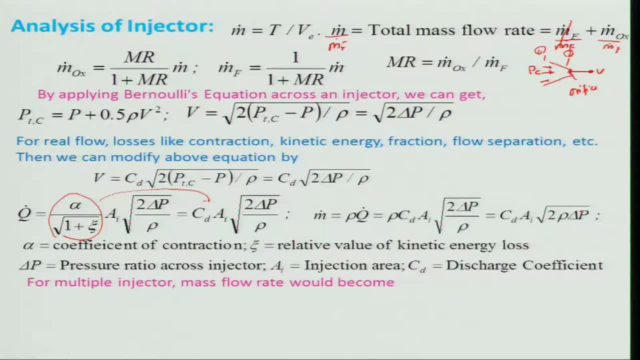 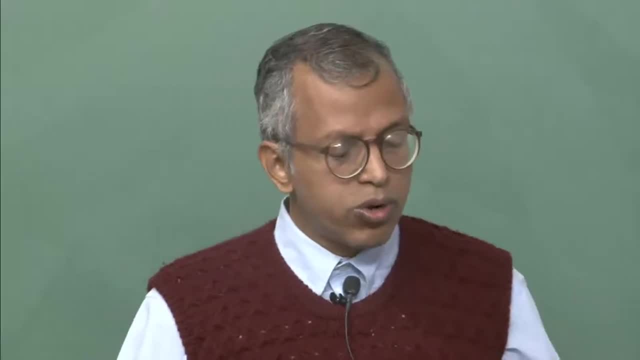 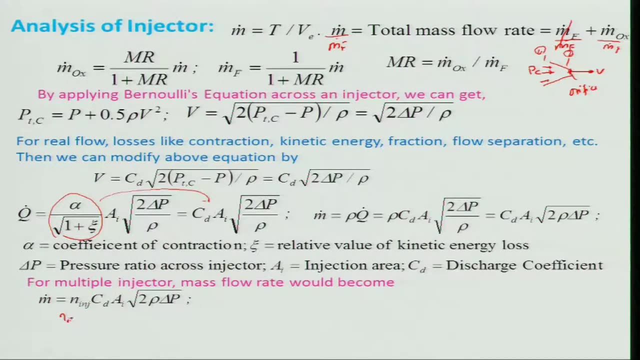 So for multiple injector there might be several injectors, right? I mean, it is in a gas, in a rocket engine we use several injectors, right? So I have already shown you how it works. it will be So. mass flow rate would be basically m dot n. i is the, n is i, n, j is basically number. 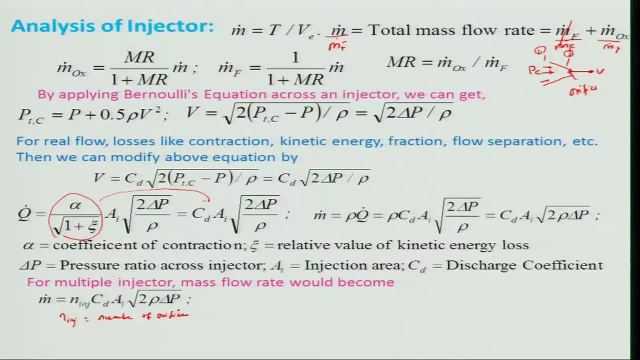 of orifices. right, how many are there? may be 50, may be 20, may be 100. you know, like any number depending upon the design And the m r ratio of the propellant became. m r is equal to m dot oxidizer divided by m dot f, which is nothing but number of oxidizer holes. 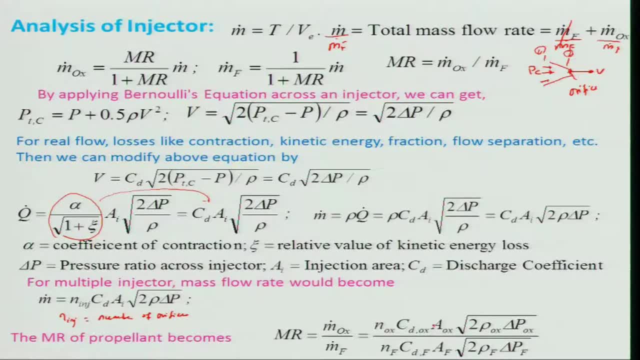 or the orifices, So into C D of oxidizer. keep in mind that C D for oxidizer may be different than the fuel. right, it may happen it may be same as well, but generally it will be different. and a o x is the oxidizer of individual orifice root over 2 rho oxidizer and the density. 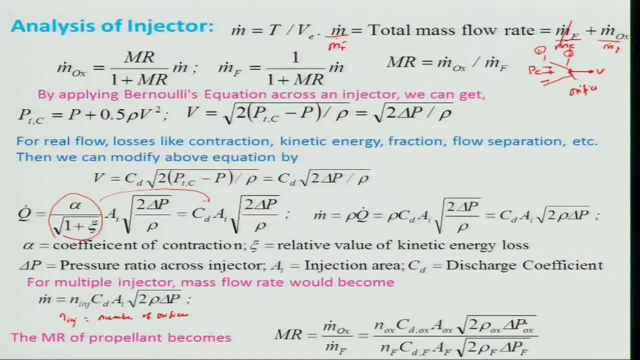 of oxygen, delta p, x, that is the pressure difference between the across the injector, oxidizer injector- and similarly for the fuel right. And if you can design this, you know values and finding out whatever you need and depending upon what- C, D and other thing, those data can be taken from experiment data or some you 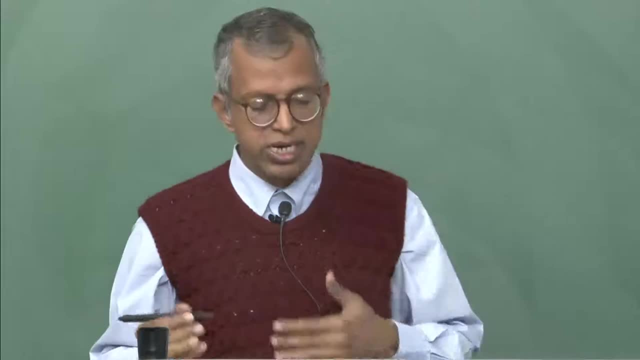 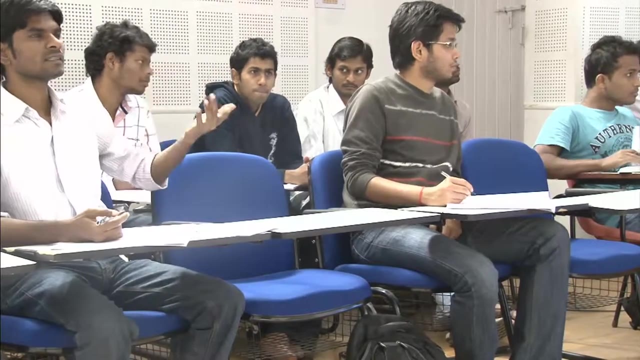 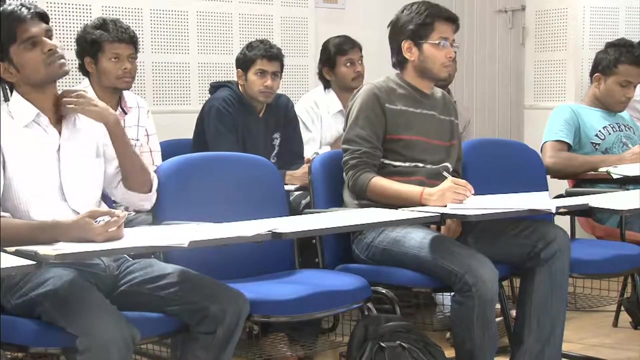 may have to design and conduct experiment yourself to find out. So naturally, because a liquid, naturally it is a liquid flow, right? We are not going to have a liquid flow, right? we are not going to have a liquid flow, aren't we? We are not dealing with gas, it is a liquid, so it will be. 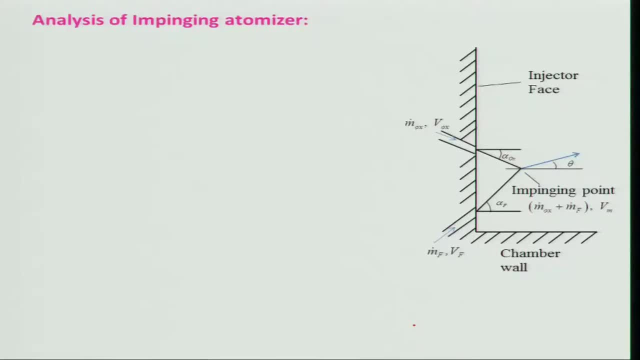 So let us look at, will be looking at this impinging atomizer. so let us look at that fuel is being atomized at an angle alpha f and oxidizer is being atomizing the alpha x. let us say that this is in x direction, this is in y direction, and keep in mind that this 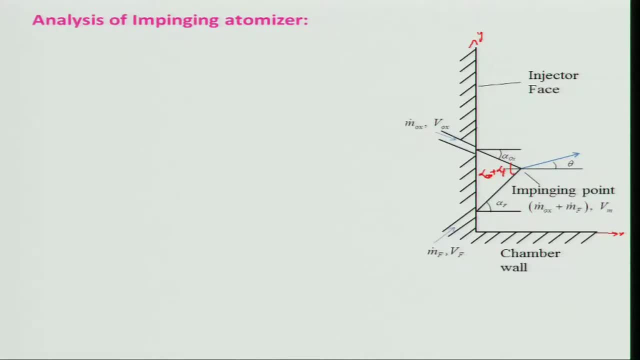 angle is nothing but alpha x plus alpha x right, and that what we call it is basically a beta right. and what we are assuming in this momentum of impinging jet is same before and after the impact. in real situation it may not, you will have some loss, but we are assuming that to be same for the design purposes. for 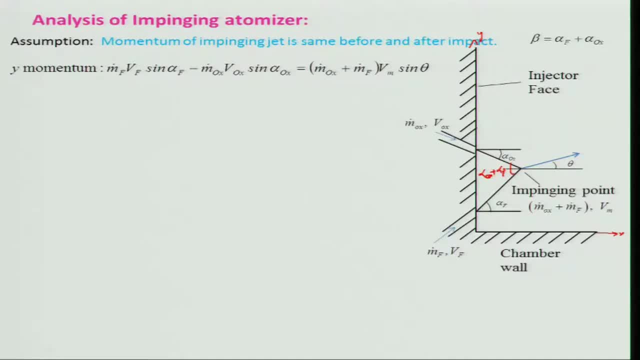 the simplicity and what we will do. we look at y momentum. what is this y momentum? if I say this mass flow rate of fuel and oxidizer, there is a two component. one is this direction and this is in y direction. y direction will be m, dot, f, v, f, sin, alpha, f, minus the oxidizer. 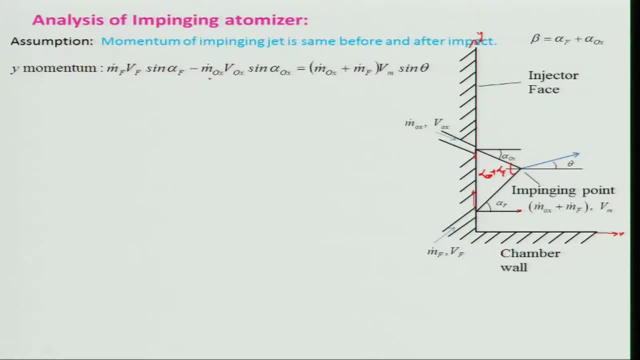 it will be in this direction, right, So that will be minus m dot o x, v o x sin alpha x is equal to m dot o x plus m dot f, v, m sin theta right. Similarly, for the x component, we can write down the cost component which I have written here right and what I will. 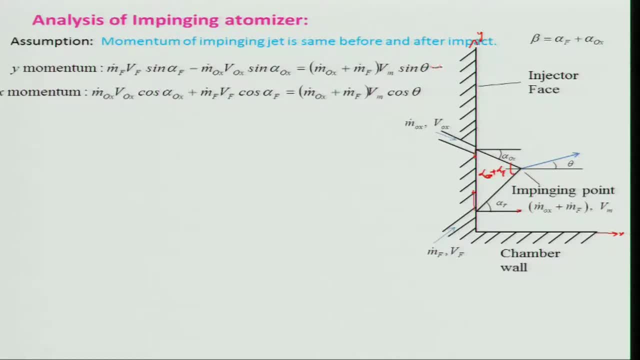 do? I will just divide this, you know, by what you call equation one, with the equation two. what I will get, I will get tan theta is equal to the m dot f, v f, sin alpha f minus m dot o x, v o x, sin alpha o x, divided by the cost component, which we have already done. that 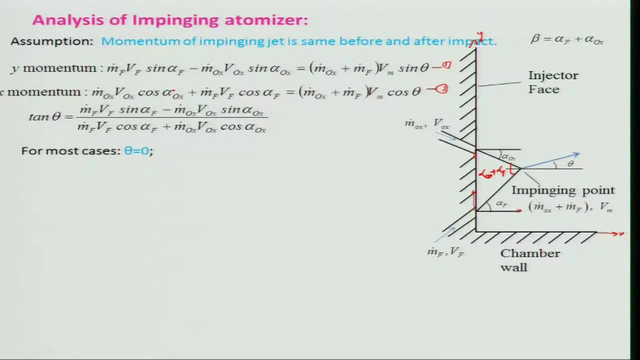 these are things right Now. if I take most cases, the theta will be zero. you know, if the momentum is fine, it need not to go with a alpha. provided if the momentum of the, both the fuel and oxidizer, same, it will be moving in this direction ideally. but however it may go, move at a certain direction. 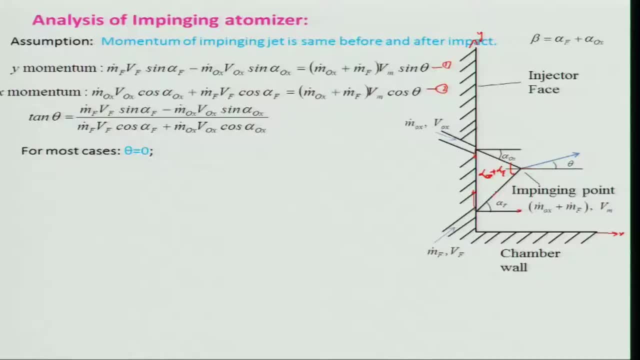 right, yes or no. So if one of the momentum is higher, it will be having this direction. if oxidizer, if the fuel momentum is higher, it will go in this direction. if the oxidizer momentum higher, it will go in this direction, any direction, but we will be assuming it to be 0.. 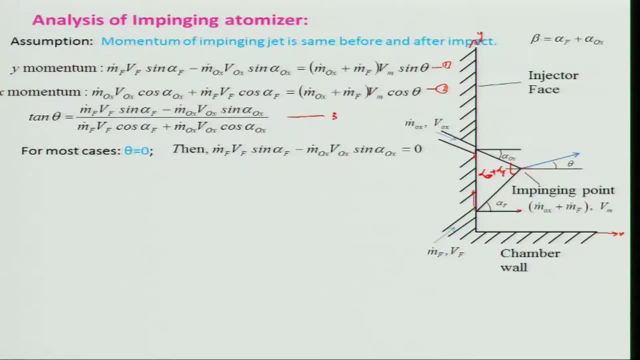 So then, what is saying that this became this expression? equation three will become m dot f v f sin alpha minus m dot o x v o x sin alpha is equal to 0.. What we will do now? we will basically look at what I will do. I will just divide this equation by m dot o x v o. 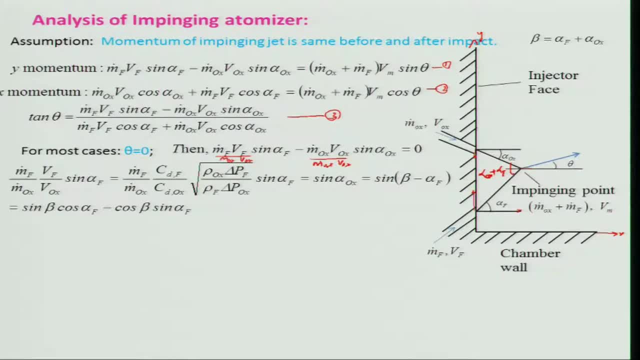 x right, m dot o x, v o x right. and then I will get this v f by v o x sin alpha x and in v f I can put in terms of T D and pressure ratio, right, that is v, for the velocity will be in terms of T D and root V. 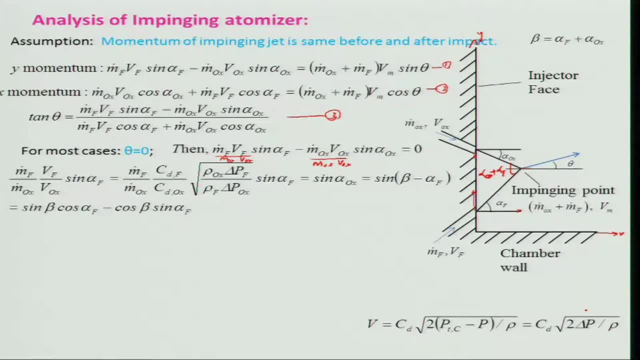 So this is what I am going to do now. I will take this equation and I will divide root over delta p by rho, So that we are doing So that delta p f by rho f is coming and 2 is cancel it out for the oxidizer. you know that one, So you will get sin alpha. 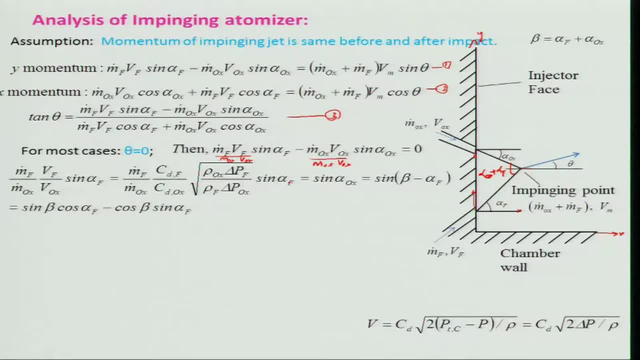 and what is this sin alpha? and the sin alpha will be coming and is equal to sin alpha o x. sin alpha o x is nothing but sin beta minus alpha x, because beta is equal to alpha x plus alpha o x. So then you can expand this sin term and then you know you will get this expression. 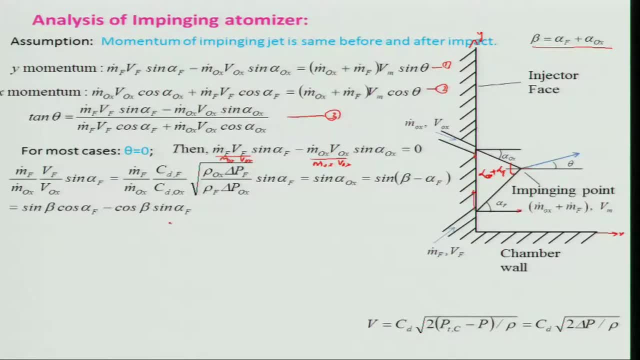 and what we will do. we will take all this sin alpha term- you know this term- to this side and we will do that. So what we will do then I will take sin alpha. f is the common, I will get this term right, this term as here: plus cos beta is equal to. 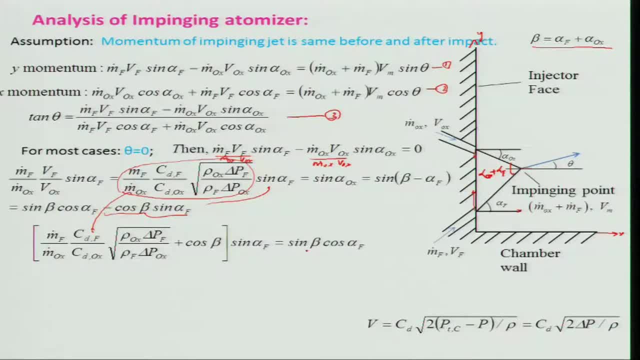 sin beta is equal to cos alpha x. Now, what I will do? I will divide by this cos alpha f and cos alpha x. So this, cancel it out, this become tan alpha f. So what I will get? I will get this alpha f is equal to tan inverse of this quantity like, which is of course 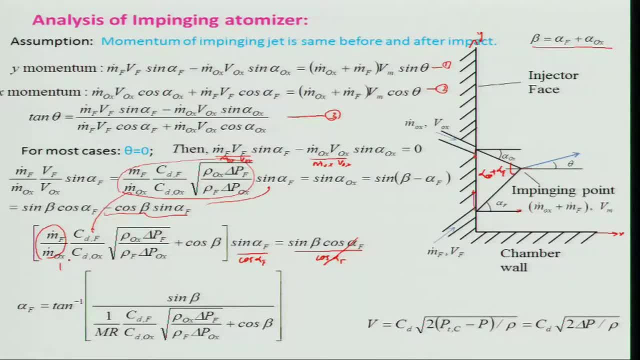 I can write in terms of: this is nothing but a here, basically one by m r. So I will write that down. will get, because if I know this beta and I know all those things, I can get what will be alpha f and alpha ox we can get very easily So you can use this as a design tool. keep. 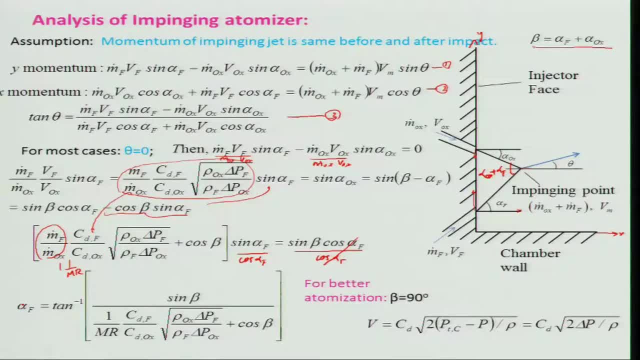 in mind that for the better atomization people always suggest to go for, beta is equal to 9.. But, however, in real situation you may not get, but you can, but this is the thing which you can use. So you can use this for, you know, finding out alpha and then other play. 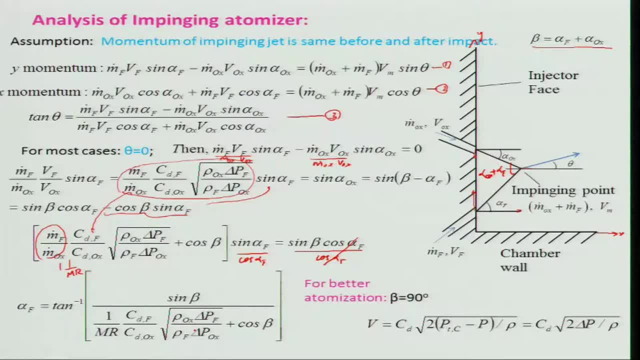 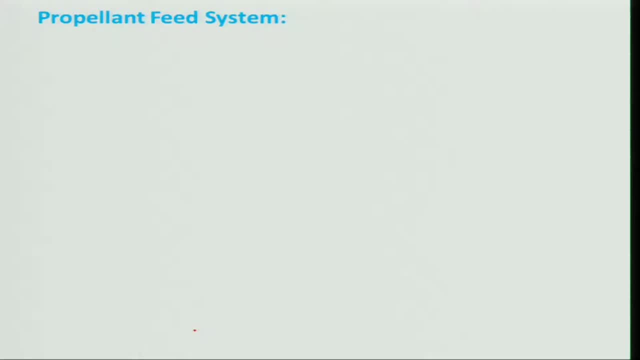 around this thing about the mass flow rate, the delta, f, e, and then look at what will be m r ratio. you can, you know, use as a design tool for this. So let us look at propellant feed system. we talk about injectors and atomizer. how to 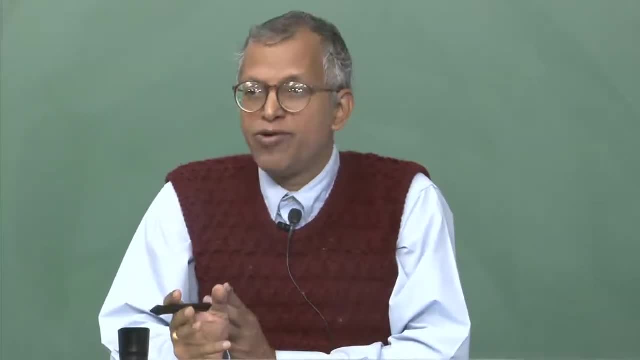 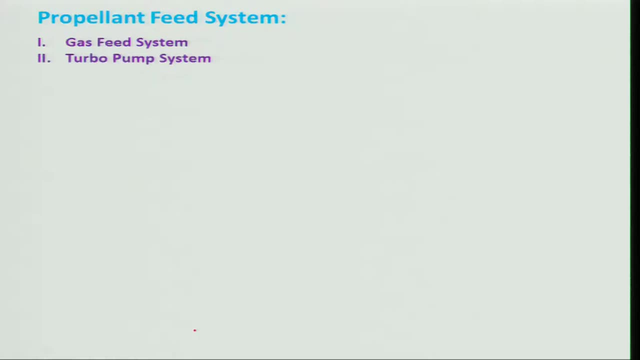 go about it, but we have not looked at how to feed this because we need to have a pressure, you know, otherwise we cannot feed. So to have it can be divided into two categories. of course there are several other varieties but I would not be discussing. 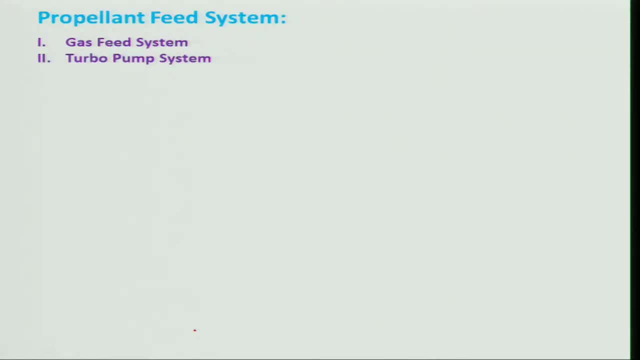 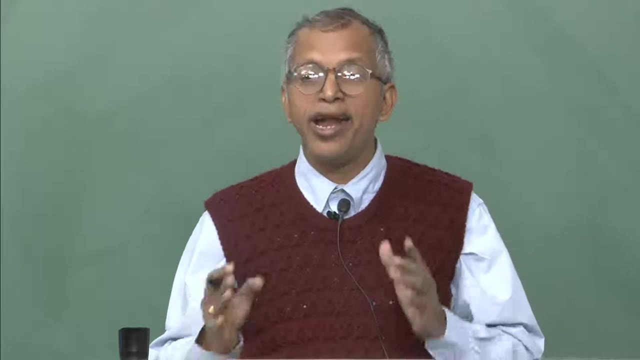 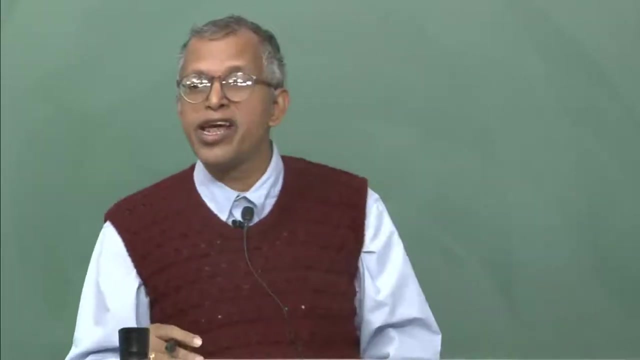 Gas feed system and turbo pump feed system. gas feed system is generally being used where the duration of the operation is small number one and the requirement of thrust is not very high. that means the pressure chamber pressure should not be very high, otherwise my overall weight will be very high. 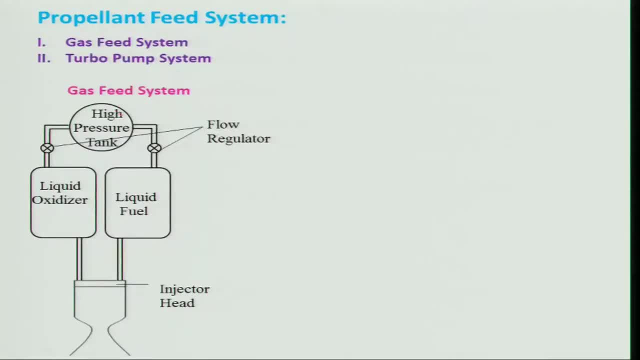 So the typical gas pressure system can be: think about a high pressure tank which contains the air Gas, any gas- basically nitrogen or argon or some other gas which is neutral, and it will be pressurizing the liquid oxidizer and liquid fuel and you do not need a feed system. this 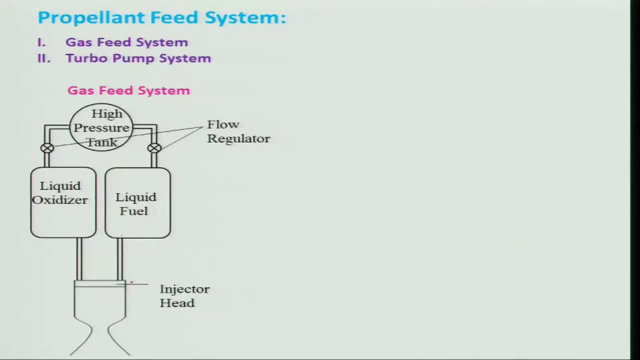 is quite lighter enough and then it will inject the fuel to atomizer and it will pass through the thrust chamber, combustion chamber, and then you will get. this is a very simpler system but, however, limitation is that the duration is very small And if- and the pressure chamber pressure should be small- you keep in mind that there is a 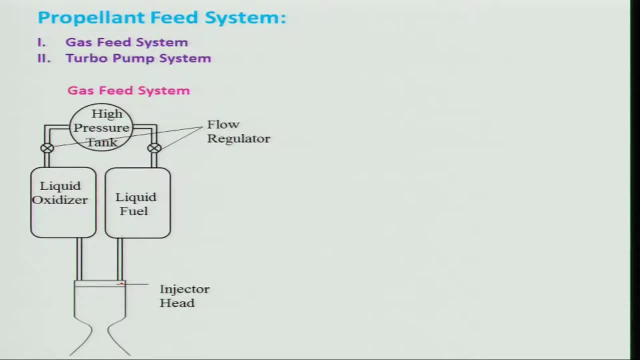 lot of pressure losses at the injector head. So therefore, you know you want to have a very high pressure in the chamber, then it will be. you know at least something two times or three times that chamber pressure you need to have in that feed line, and then you will have to go another. you know very higher level. 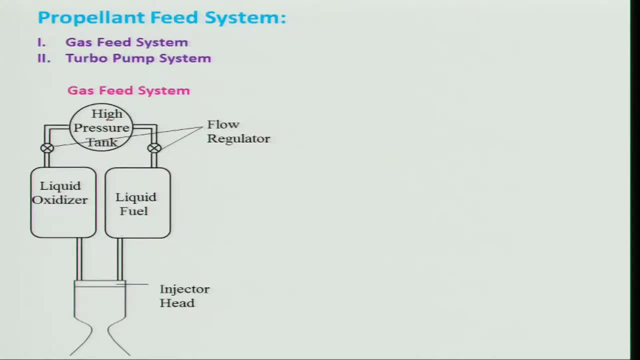 of four or five kind of things. high pressure tank, Right. So therefore it is being limited, but in order to, and then time duration should be small, otherwise you, your tank, pressure tank will be very high. you know, otherwise you cannot operate But to in order to overcome that problem. so what is being done is that you use, we use. 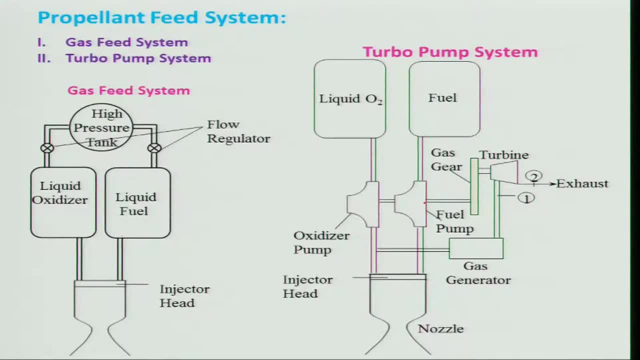 a pump, the pump for the oxidizer and pump for the fuel, and to run this pump which we need to have a turbine, of course, through the gear box we can use that. I mean you can reduce the rpm of the you know so that you can get a better efficiency in that. 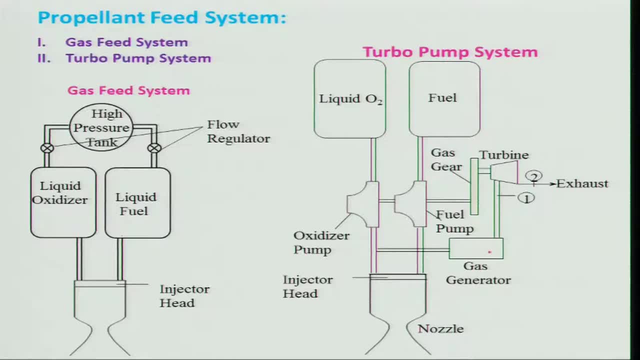 And to run the turbine we need to have a gas generator, another combustor. that is a very important thing, Otherwise how will run it Right? So this is being used for a long range and for a very high thrust level, kind of thing. what I will be showing now you discussing about three types of turbo pump system. 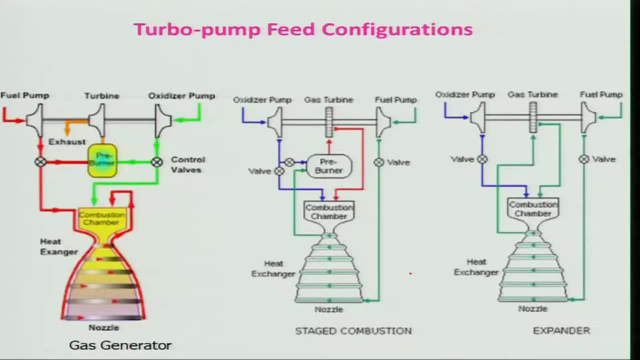 Right, There are three types, but there can be several other types as well. one is gas generator. one, if you look at it, is having fuel pump and oxidizer pump, which is run by the turbine Right And in this case the fuel, you know, being separated. one line goes to the pre burner and other 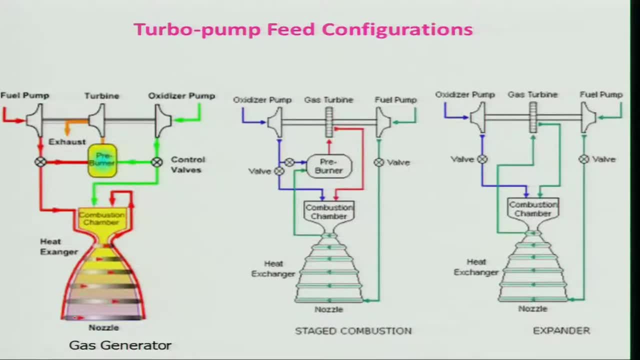 line goes to the what you call rocket engine, which will be cooling, and then it is injected into combustion chamber Right And whereas the oxidizer, again divided in two stream by the control valve, one is the burning, you know burners, pre burner for the turbine, which will prepare high pressure, high. 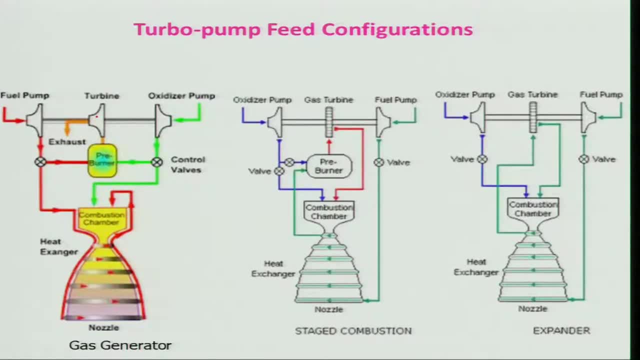 temperature gas which will be expanded in the turbine, And these turbine will be expanded till the pressure, ambient pressure. generally it will be low Right. In the particular, when you are operating at the high altitude, Then the pressure ratio is quite high Right. 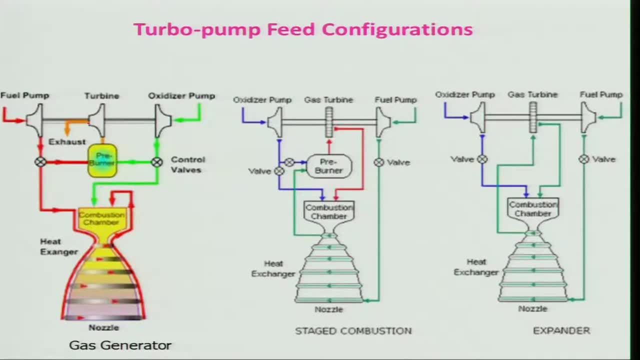 Then the number of stages, you know requirement will be more and if you go for more number of stages, then the weight will be more. of course you will get a higher. Therefore, this pressure, operation, operating pressure for this pre chamber is being, you know, very, very low being used. 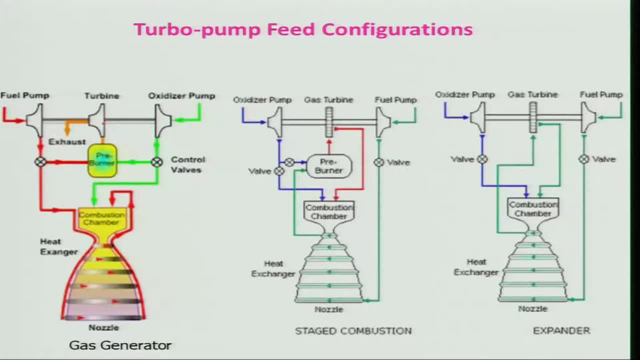 And as a result, then the chamber pressure, if it is not operated, you know, at a high and the work is not more, then you cannot have a high pressure in pump the chamber pressure which is being limited to Right, You know low pressure. generally people talk about something 5 mega Pascal kind of things. 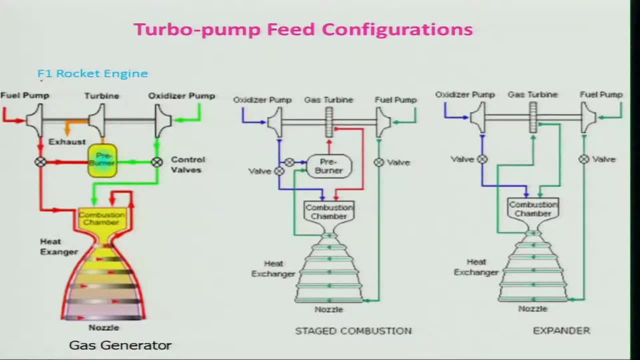 and it is this kind of system is being used in the what you call F 1 rocket engine. The most, which is used for the for a high or the high thrust rocket engine is known as stage combustor. If you compare the stage combustor you know it is with this gas generator. it is the same. 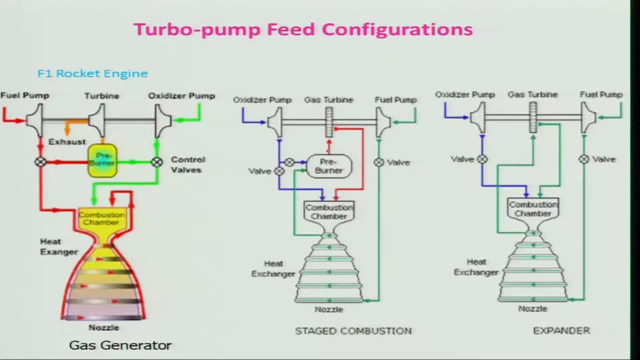 only difference is that only difference is that You know that high pressure gas, temperature and gas which will be burnt, will produce in three burners is being expanded till the pressure, whatever it is required. That means after it is getting expand turbine it will come into the combustion chamber and 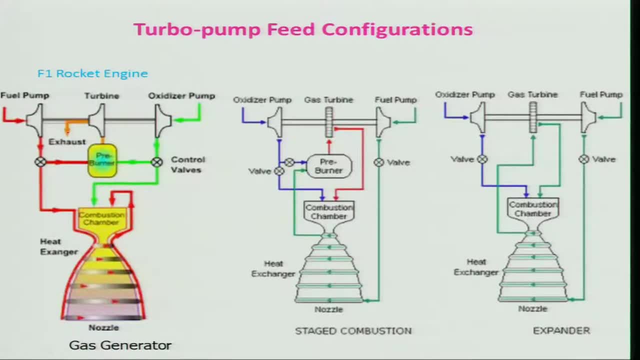 it operates And here it was a loss because the fuel, some of the fuel, or high temperature will be there, some of the this thing here you need not to operate at a. you know this thing and you can operate this combustor at a high temperature. 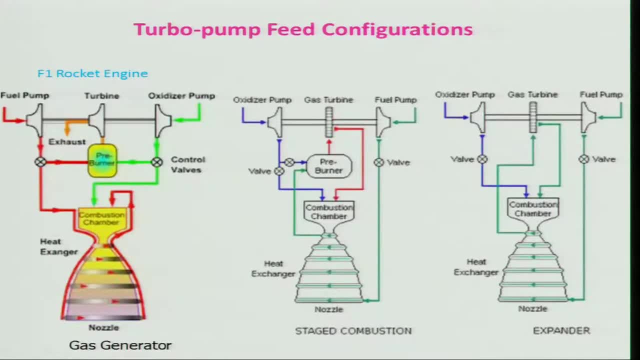 Right, But also a fuel lean. some of the fuel can be utilized here. as a result, you can operate at a very high pressure. this chamber pressure right, combustion chamber pressure, or the thrust chamber pressure, which is order of 50 mega Pascal instead of 5 mega Pascal, kind of thing. 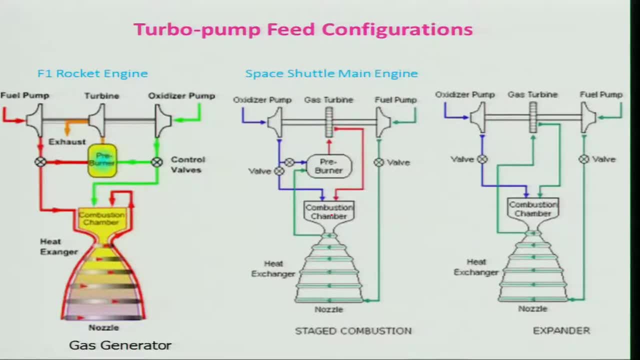 So that is being used in space shuttle main engines. you know it is being used. of course little modification is there, for there it is a fuel and oxidizer pumps are separated is there to the same gas turbine. but this is being separated right, So the another one which is being used- the complexities of three burner- is not there. 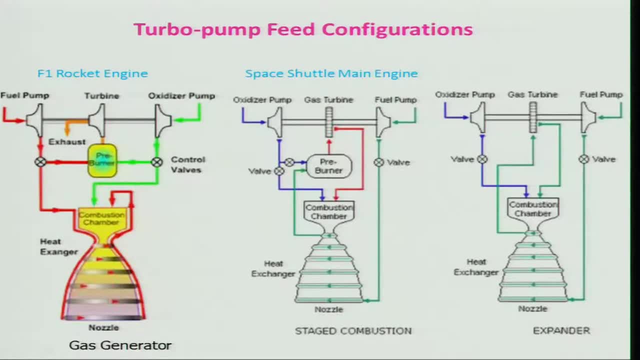 rest is similar to that of the stage combustor. but problem here is that, like you cannot really get a very, because when the fuel will pass through it is not having, you know, very high enough pressure to operate in that to that. So therefore very less amount of pressure you utilize in the gas turbine because you 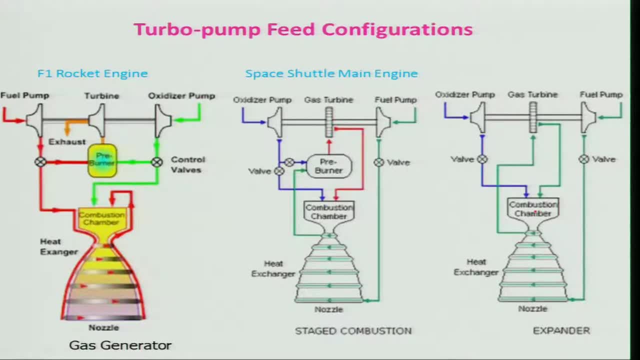 will have to operate and therefore this is being used for the small rocket engine where you know the pressure chamber, pressure restricted to around 2.5, 2.7 mega Pascal, kind of thing. So that is being used. R 10, you know something? liquid oxidizer, liquid in several other places. 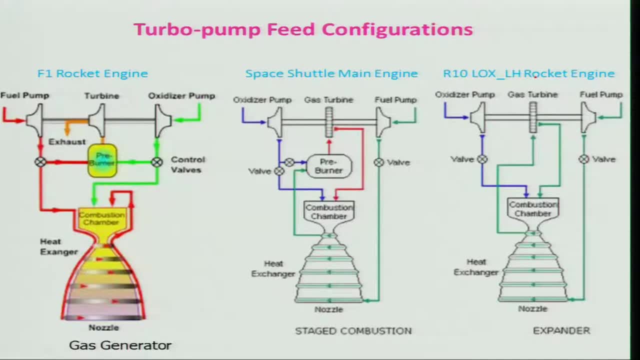 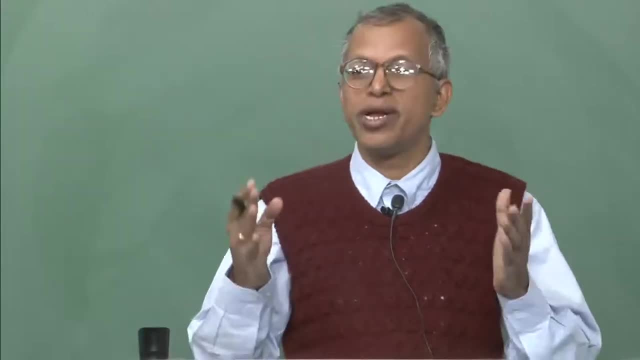 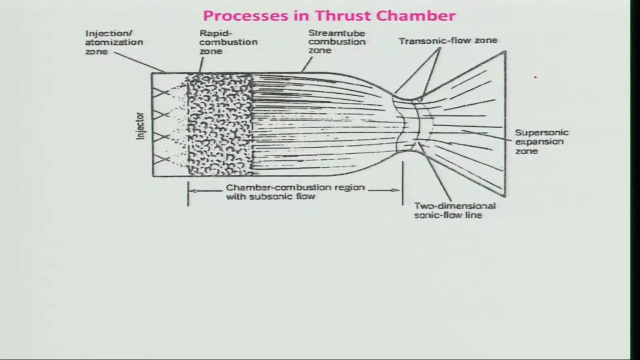 So this is not that you should not think these are the only three, but there can be several varieties depending upon your requirement, depending on your mind, depending on your creativity to meet the demand. that is the beauty of the engineering work. So let us look at what is happening in the processes in the thrust chamber right. 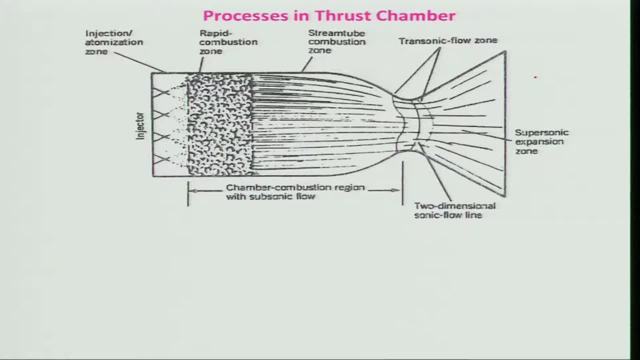 If you look at, we have seen the rocket engines- and then it can be, you know, like injectors head are there here and it is having, you know, like a two phase flow kind of thing. heterogeneous right mixtures will be there and there will be also the velocity with which it will be. 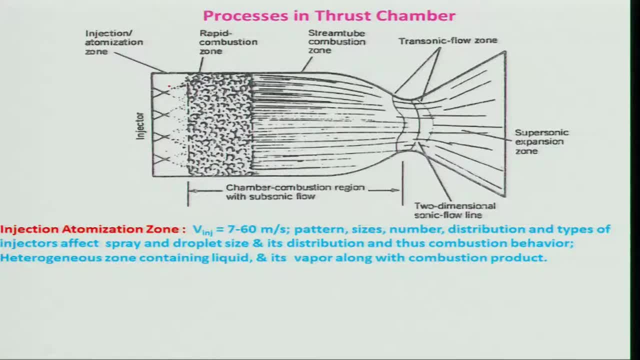 flowing. So the velocity is something 7 to 60 meter per second and, if you look at the combustion behavior, will be dependent on the spray quality. Spray quality will be dependent on injector pattern, sizes, number like number of injectors or orifices- distribution and type of injectors. what we- because we have seen several injector- 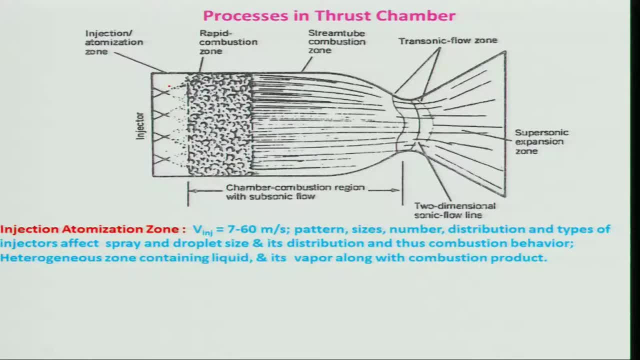 types you know, and then the combustion behavior will be detected. So therefore, this is a very important part for the thrust chamber. So you have to have this, but thing is that it will be having heterogeneous in nature. there is a liquid phase, vapor phase. vaporization will be occurring right, and also some of the 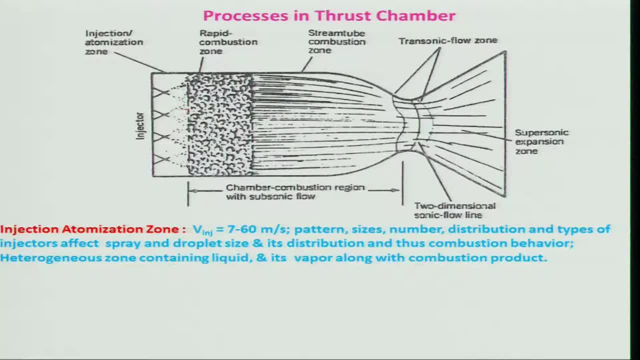 combustion, which will be coming into this places also because particularly in this zone, right. So therefore, some kind of thing and may be some reaction might be taking place, but it would not be releasing any amount of heat. that is known as injection atomization zone. 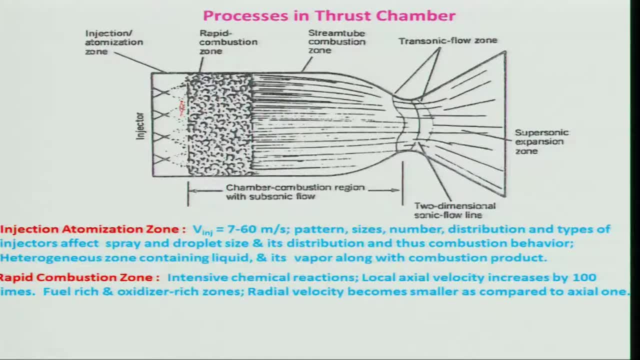 There is a rapid combustion zone where intense chemical reaction takes place and the local heat will be increased by 10 times. For example, if it is 60 meter per second, it will be going to the you know very, very high velocity: 7 meter per second. it will be going to 700 meter per second right. 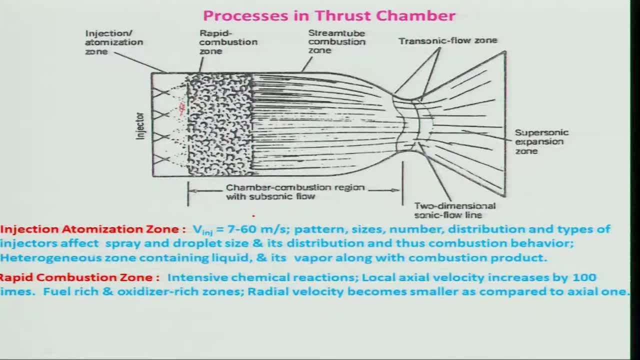 But however you know, it is a order. it may be go to 50 times as well, you know. but general, you know it will very high. So there might be fuel reach zone and oxidizer reach zone will be there and the radial velocity. 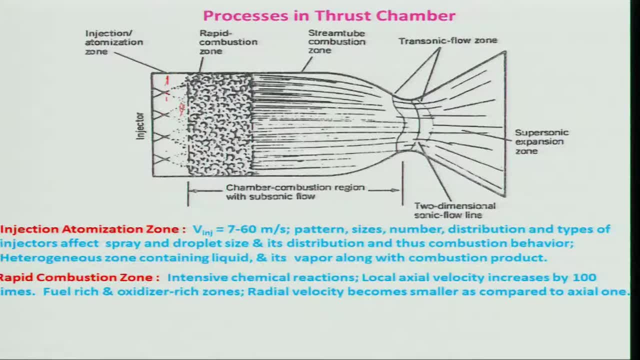 because here it is impinging, the radial velocity will be there along with the axial velocity and might be tangential if it is fluid. Here the radial velocity is more and the very, very less, and the axial velocity will be very high, and then you will get a what you call very high velocity region. 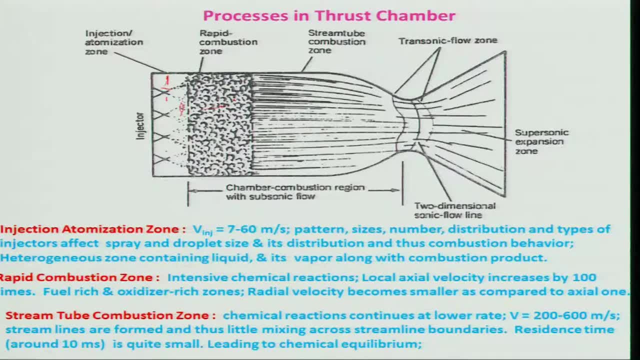 And particularly in this zone, reaction taking place, but in this zone reaction will be reduced. that is known as stream tube combustion and a zone where steel combustion will be taking place. It will be reaching, going towards the what you call equilibrium position. and but how? 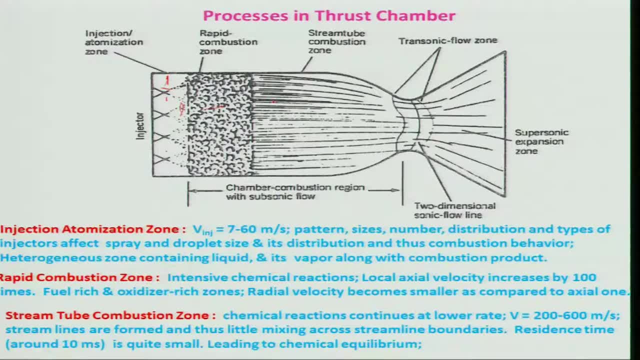 ever. the radial component is very small, negligibly small. therefore it is a stream tube. there would not be any mixing between this tubes or the stream lines, you know, tubes, And the velocity, which will be order of something 200 to 600, even more meter per second, and 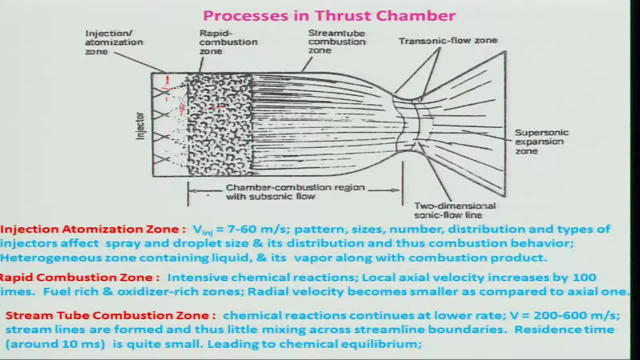 some combustion will break in place and this zone where you know subsonic regime, will be there. Subsonic because velocity is very high, because the temperature is high, therefore it will be subsonic. So and this zone, it will be expanded and some of subsonic will be there. 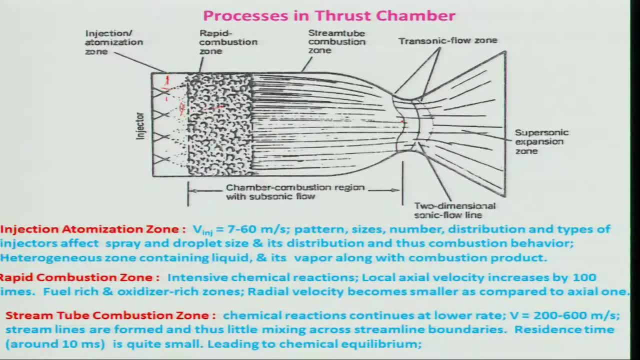 Sometimes some of the combustion goes till the throat area, right, but that will be very, very negligible. it should be So. if you look at it is a quite a complex process. you know that amount of time, residence time for this is order of some milliseconds. you know 10 milliseconds, 7 milliseconds, 15. 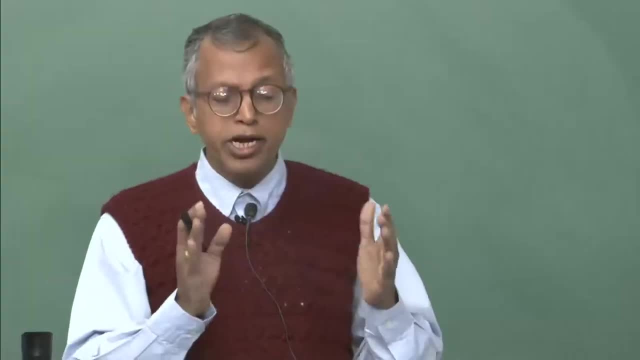 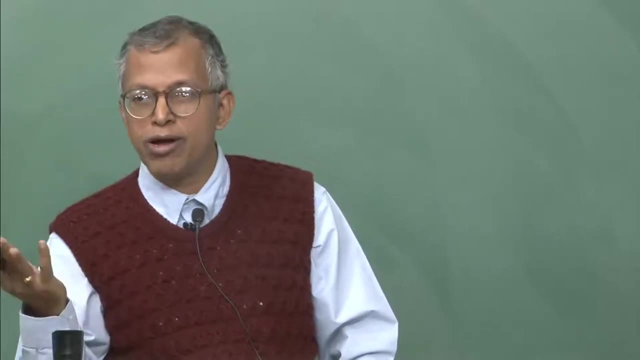 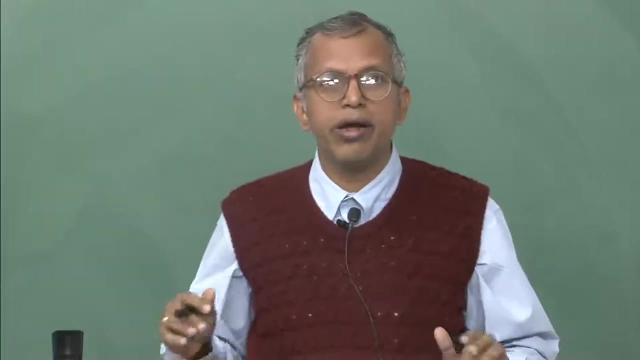 milliseconds, like kind of thing. So therefore it is a very intense combustion takes place. as I told you, the amount of heat release in the rocket engines is much higher as compared to the, you know, gas combustion. gas turbine, particularly per unit area, I told you, is around, say, 370, kind of things you know. 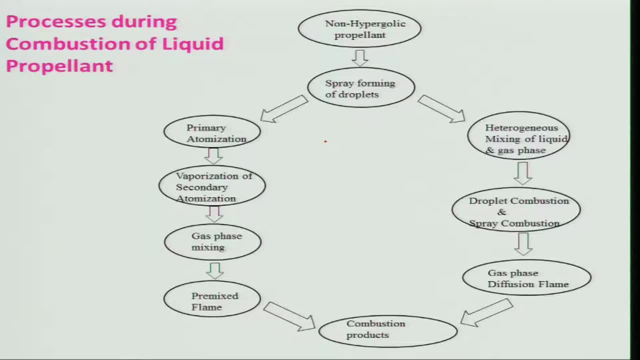 mega joule per meter cube. So let us look at what is really happening in combustion zone. So the I will talk about two kind of thing. one is hypergolic propellant, that is, spray forming of the droplets right. non hypergolic propellant and it can be having primary atomization. 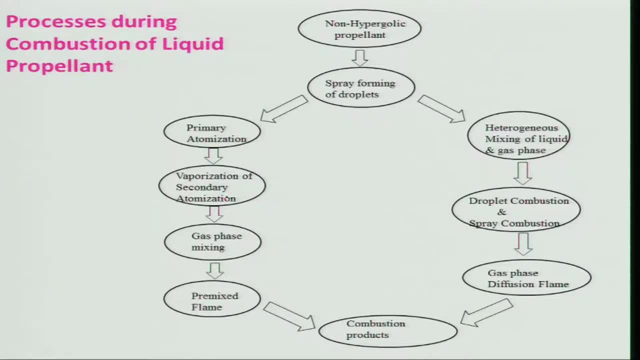 And then when primary atomization occurring, then vaporization of secondary atomization can take place right, and there might be a gas phase mixing. So vapor has come. then, you know, fuel and oxidase can mix and it can lead to a pre mix flame, right, some places- it is not that all the places- some places there might be a pre 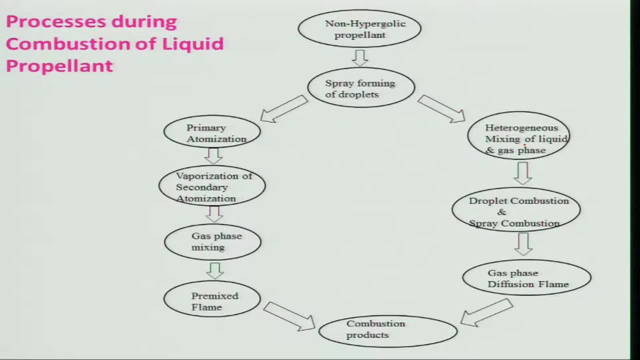 mix flame. There is another route. heterogeneous mixing of the liquid and gas phase can take place and there might be a droplet combustion. right, I will show you in the next slide. there might droplet, there might be spray combustion and sometimes the group combustion. you know like. 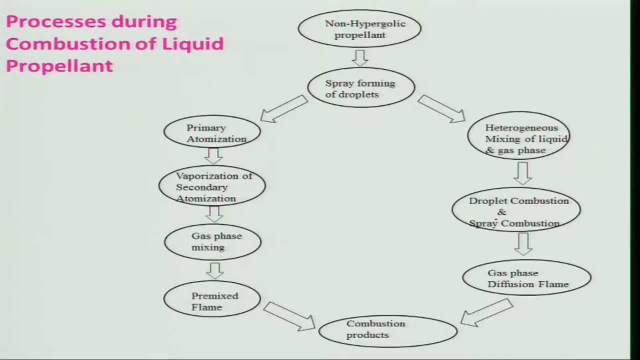 several droplet will be together, will be boiling Right and two droplet will be interacting each other. you know, anything can happen. then there will be gas phase diffusion. flame also will occur, So there is a combustion. So if you look at it is a very quiet, complex, whatever we have learnt, you know diffusion. 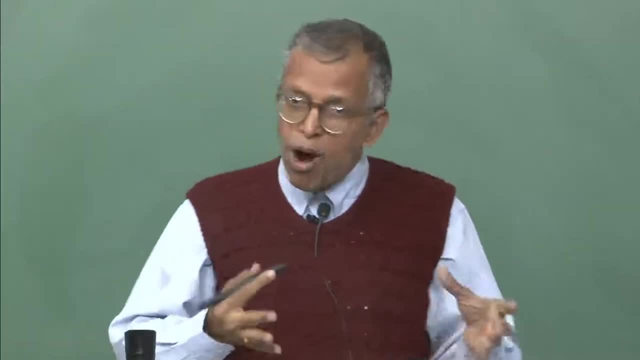 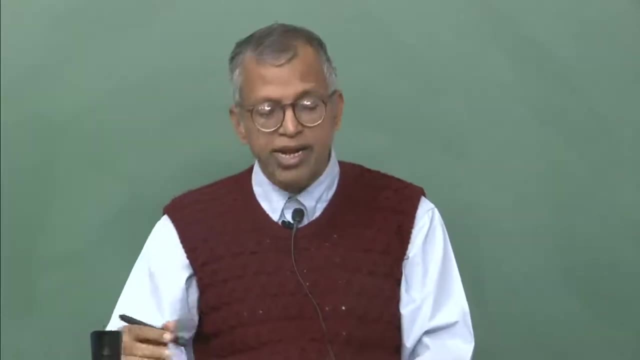 gas pre mix flame and then partial pre mix flame. all will be occurring in various places, So it is very difficult to say what is happening inside and which is not being understood really till date. So let us look at hypergolic propellant. the mixing in liquid phase will take place and 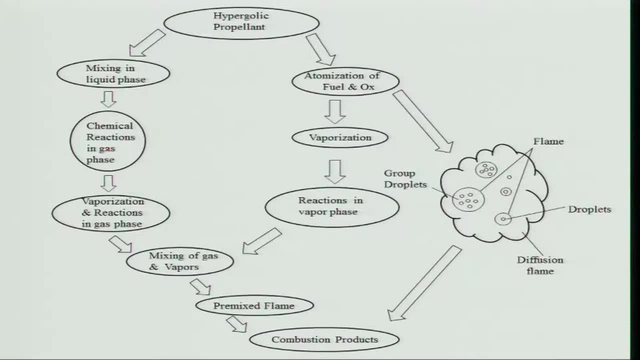 chemical reaction in the gas phase. you know one is likely to occur because it is a hypergolic in nature. So vaporization reaction in the gas phase also will be occurring simultaneously. see this, all processes, whatever I am describing, will be occurring simultaneously, not that 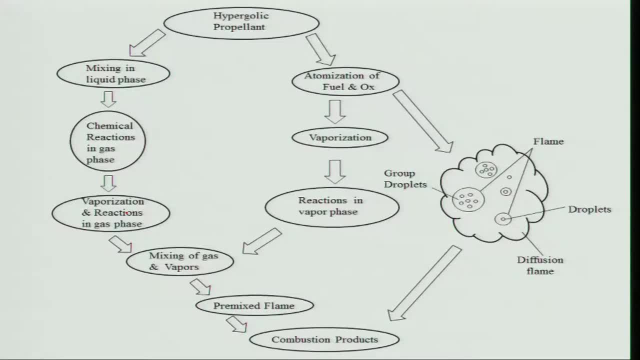 one will occur like that way: arrow is given no right. So then mixing of this gas and vapor, and there might be atomization of fuel and oxidizer. there is a vaporization and a vaporization occurs, it can mix Right, And there might be a vapor phase reaction or the gas phase. vapor means basically gas. 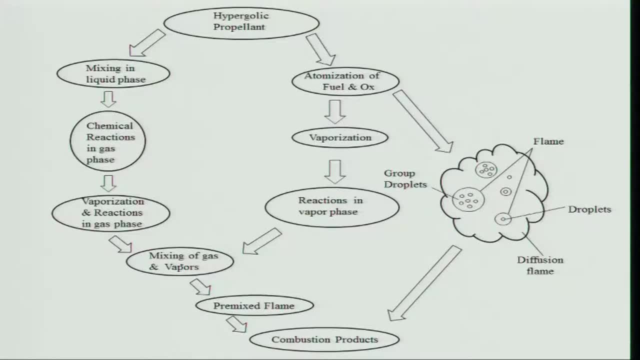 phase reaction and then this, some of this vapor will be also mixing with the liquid or the product, and then it will be, it will leading to the pre mix flame Right. There is another route, which is only the atomizer there might be. these are the group combustion. 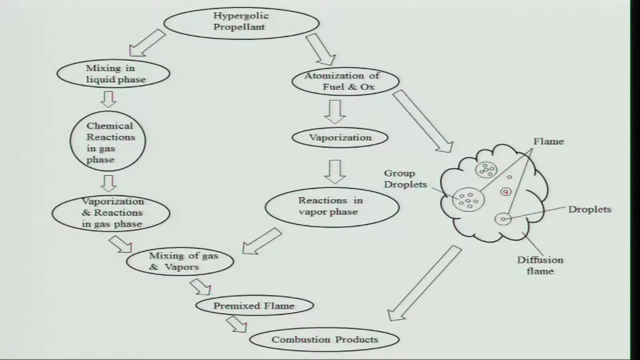 what I am talking about, and this is the flame, you know, and there might be a small droplet, there might be another droplet here, you know, it is a kind of thing which will be there, Right, There might be one droplet here and another droplet here. you know like it will be occurring. 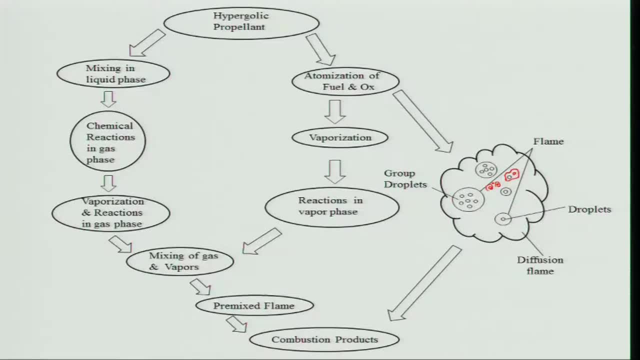 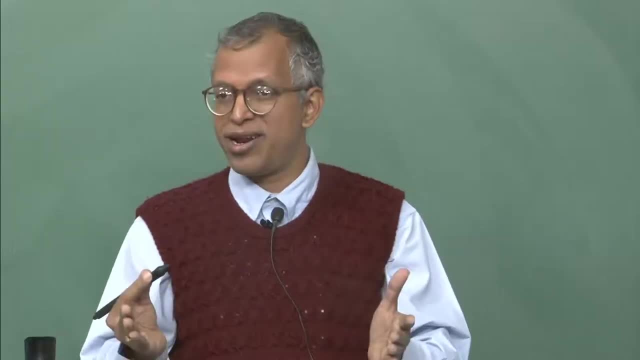 So any complexities, it can happen. any permutation combination can happen. it is random in nature. So therefore the combustion product will be getting, which is quite complex. it is not easy to model, it is not really easy to really even look at in experiment. 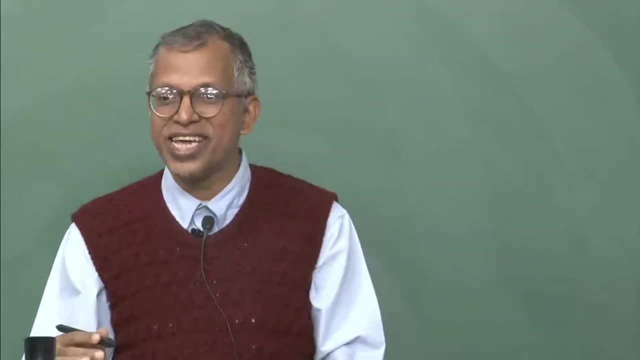 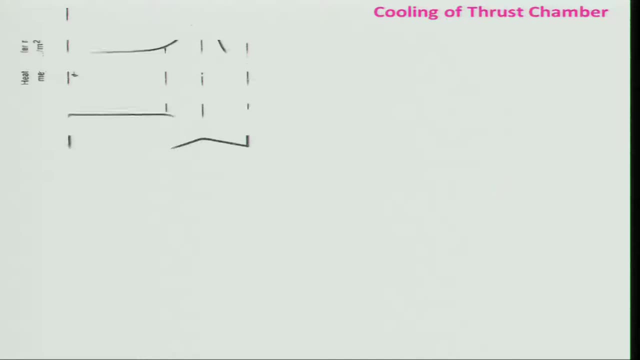 But system is working, but we have not understood what really is going inside. So with this I will. what I will be talking about is one is the cooling of the thrust chamber, which is very important because, if you look at, lot of heat is being generated. 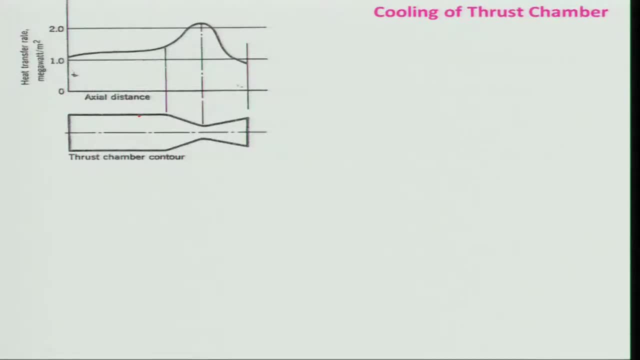 here And, as I have told you that the amount of heat being generated is quite high, it is order of something: 300 mega joule per meter cube, and the heat losses will be there to this zone. And keep in mind that the material you know is not there to withstand high temperature. 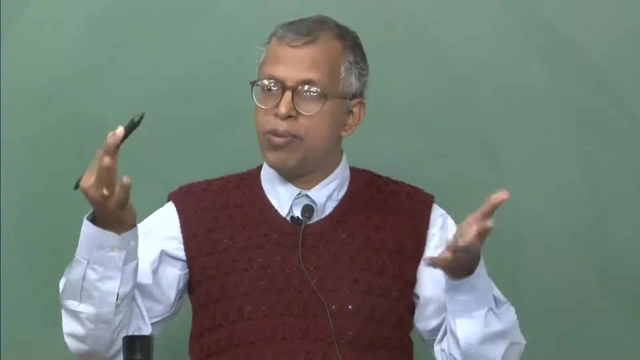 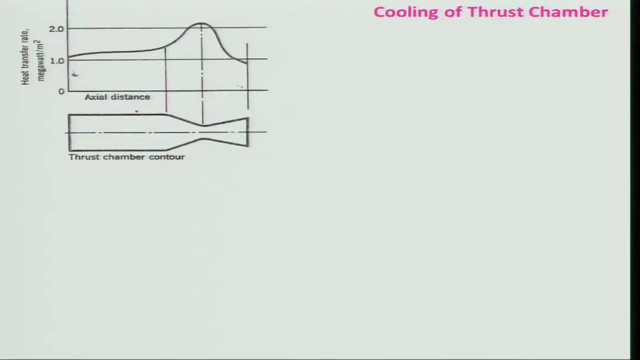 because very high temperature and high pressure pressure is order of 100 bar kind of thing, you know, 50 bar, 60 bar, 100 bar like that. So therefore the material has to be cool to have a. you know, take care of this under. 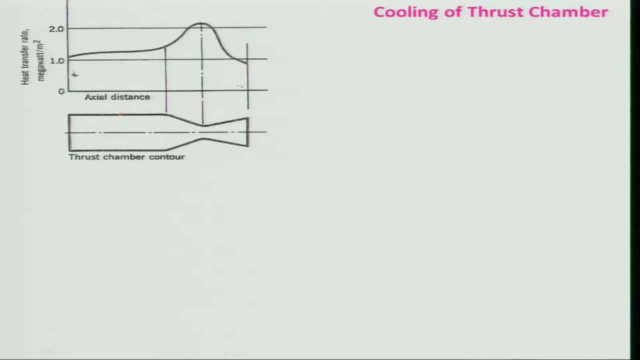 high pressure temperature, otherwise it will fail right. So therefore heat losses or the cooling of chamber is very important. if look at, the amount of heat transfer which is occurring in these zone is very, very small in the length of the combustor. along the length it goes on increases. 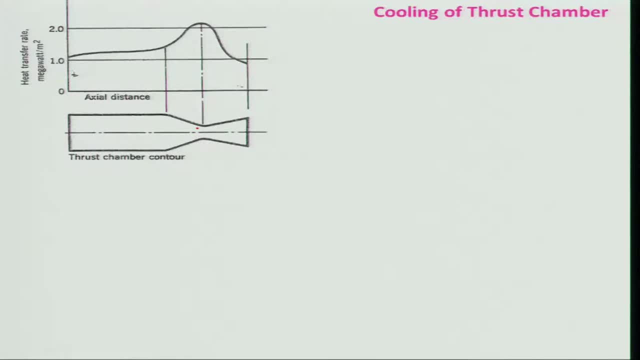 And it become peaks at the throat area. throat area is most vulnerable part of failure because the almost two times or more than that what is there in this zone. So there are several. you know methods which are being talked about. one is regenerative cooling and film cooling, transpiration cooling and ablative cooling. 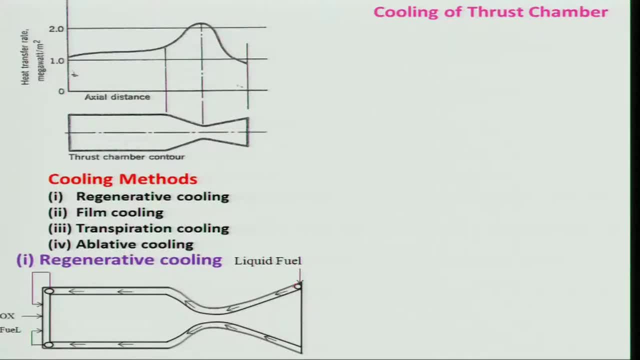 So let us look at regenerative cooling. what happen generally? the liquid fuel is being used which will take the heat and then vaporize, So that you know this portion. So this is the process of the cooling. you know, like wall will be at a lower temperature. 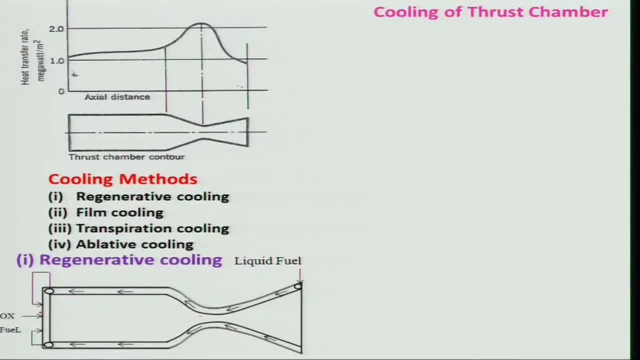 of course there is another way of doing is that you can, you know, reduce the heat losses to the wall by having a reach fuel here in this zone, So that you know heat would not be going. is like a insulating act. that is, of course. 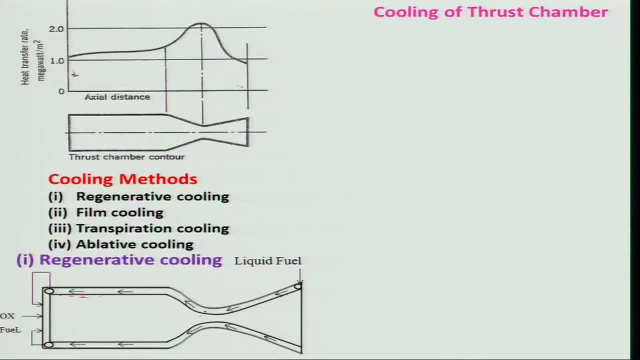 one can design And it is being used in your cryogenic engines very much, and then liquid rocket engines also. but there is a problem with that Because losses will be very high. and I think there is another cooling which is being used- is known as film cooling. 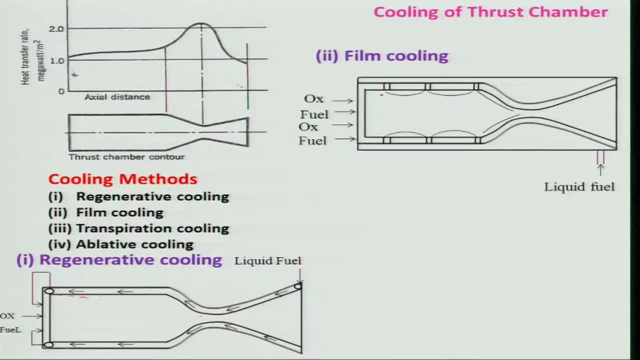 In the film cooling what will happen? there will be small hole, So is the hole will be here in the in the similar way, across the whole circumference, and it will create a film like insulating layer between this combustion zone, which is at higher, and between the metal. 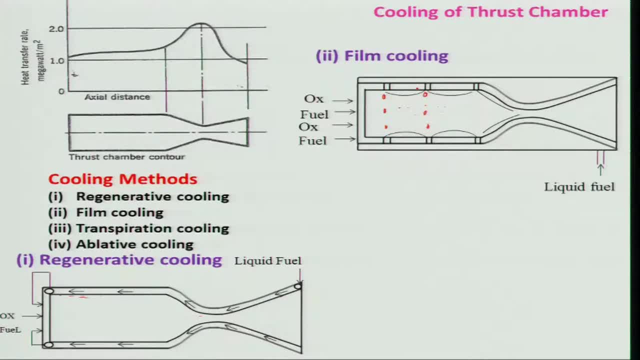 And this film is very important and it is having a length which is has to be, you know, very, very small distance has to be maintained, otherwise it will be destabilized And then it will be also oscillating because of flow will be very turbulent and other things. 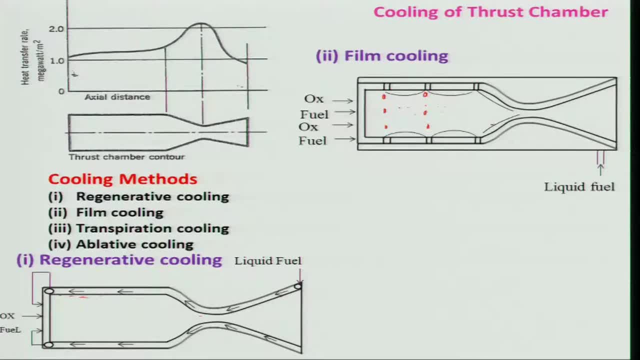 So mixing will be taking place and it will be. if you look at, the number of film is very much and 10 percent of the liquid we can give. otherwise, you know, it will deflect, it will be participating And it is a loss in, you know, because it is not participating in combustion. it will be. 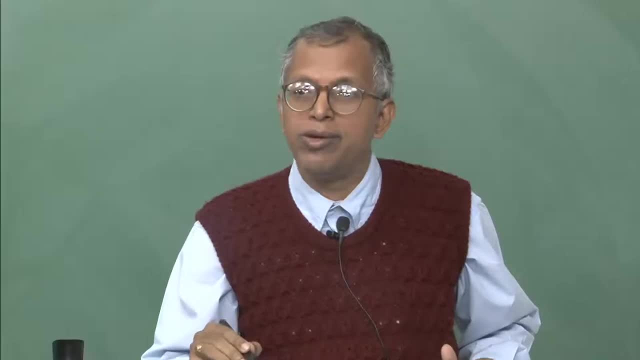 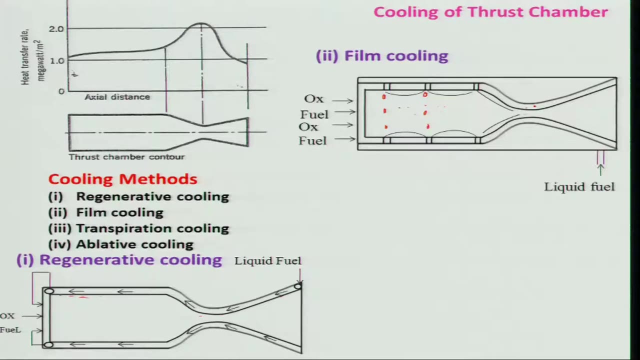 acting like a insulating layer. So the ISP will be going. And another important thing, that in the nozzle it is a very high velocity in the throat. you cannot really cool it, which is a very important one. In order to overcome this problem, of course, one idea is that known as sweat cooling. 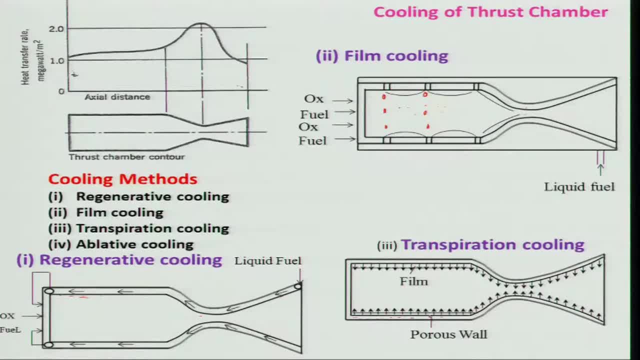 That is, you use a porous, you know material and then pass through this liquid right, such that it will be having a pores and it will be very, very low velocity. a film will be created. you know, film is not like that way I have shown, But rather a film. 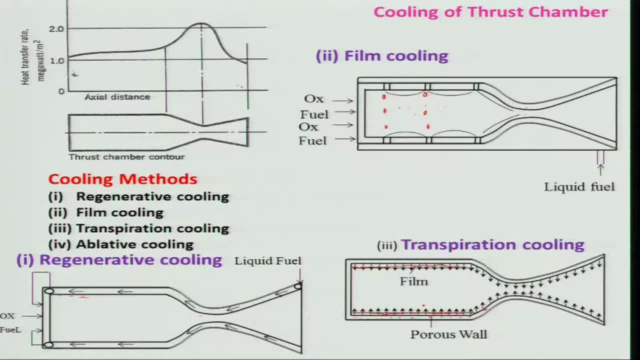 A film, very small layer, and here in this case instead of 10 percent, you know, generally 1 or 2 percent of fuel or the liquid will be giving, So that it will be good enough to have that, but unfortunately, because of material, you know, it is not being used very much. it can do any portion, even including nozzle. 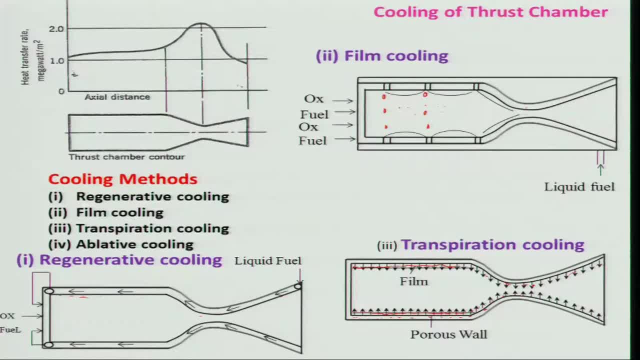 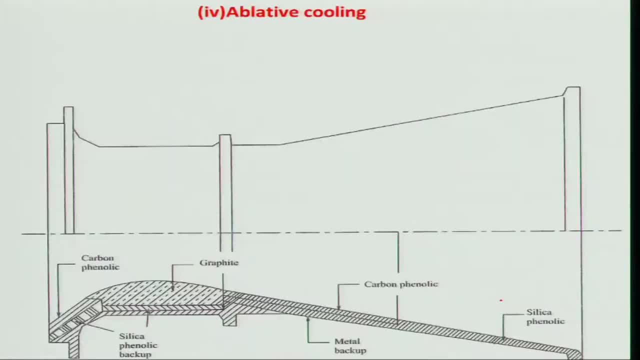 So that is the challenge: what is being, but experimentally, people are working on this. There is another one, which is ablative cooling. right, and this is ablative cooling. what is being used is basically at a high temperature, it will be converted into a char and liquid. 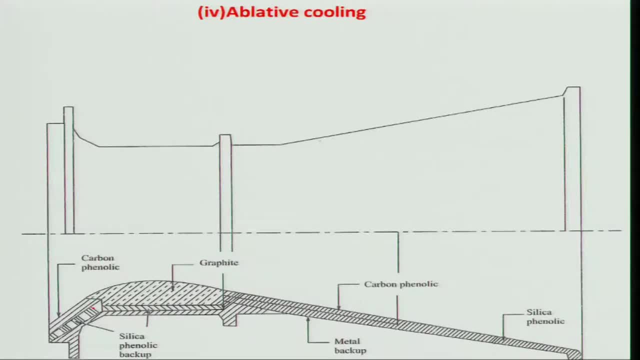 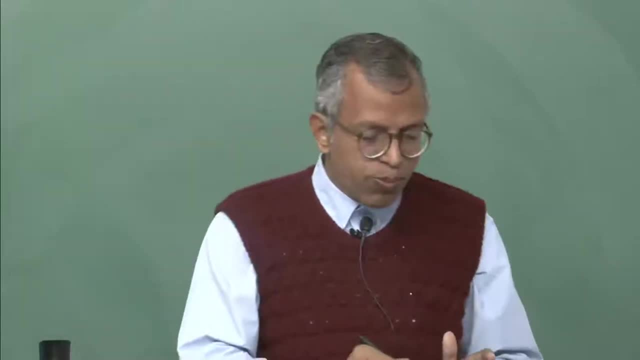 or a vapor, you know, depending upon what you are using, and it will be receded. but those material which will be remaining is act like a what you call insulation, So that it would not allow the heat to pass through the metal main metal right, and this 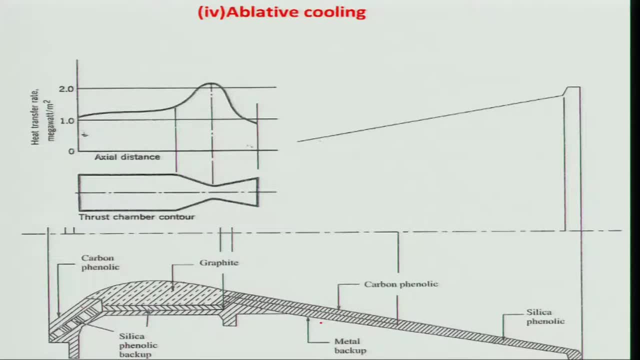 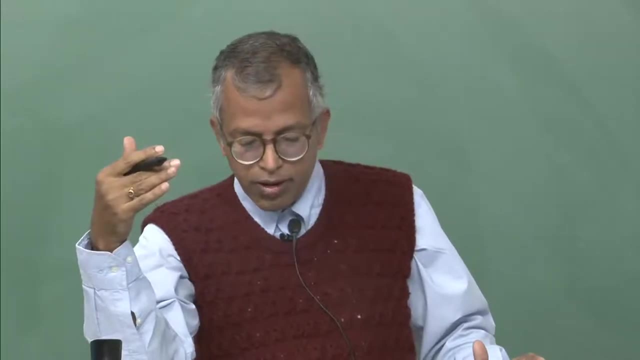 is being used, particularly in the nozzle region, other places and there is a two. you know there are several ablative material But the carbon phenolic and silica phenolic which is being used, you know, because it is having higher ablative temperature, particularly the silica phenol, is having little better. 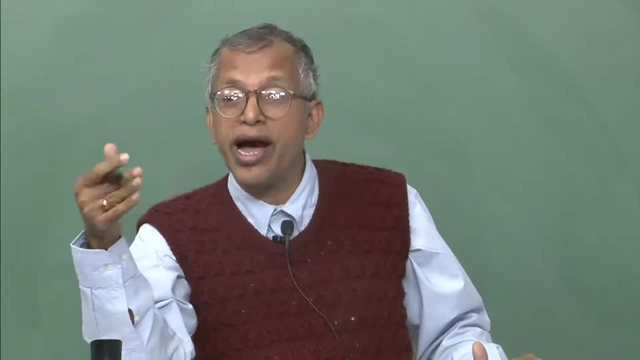 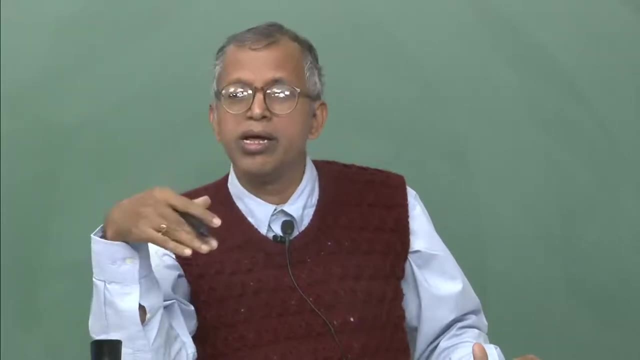 particularly because it is insulating. properties are higher as compared to carbon. and then temperature, whenever it reach 1400 or 1500 Kelvin, depending upon your material, then you will start ablating. ablating means it will be receding, vaporizing So that it will cool that thing. 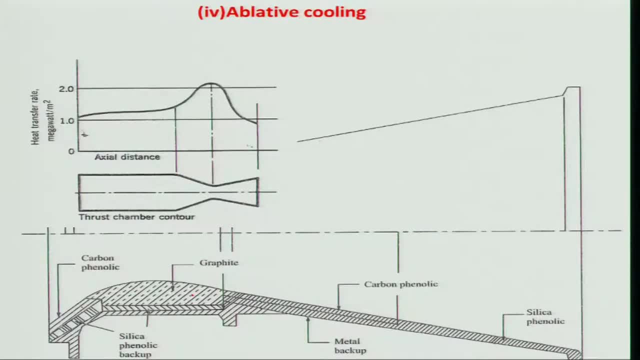 And of course, the throat region is very, you know, very- high and if it will reduce because of this ablative, then there will be a problem. for that we use the graphite, high temperature graphite, So that it will be take the high temperature and also, you know, some of the heat act like 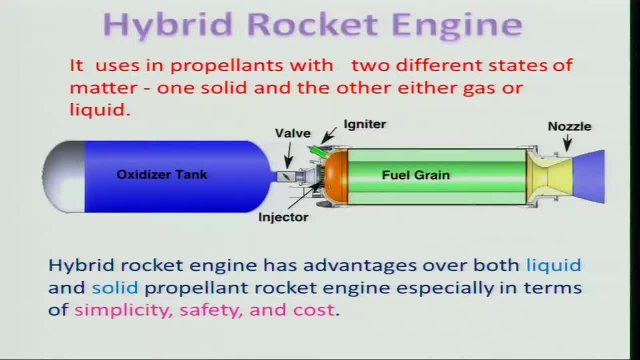 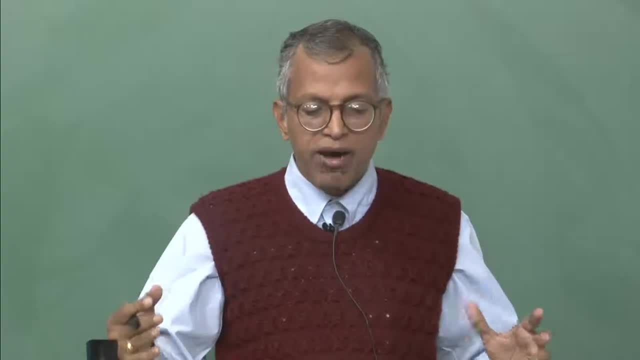 insulating, So what you call. we will be now looking at the hybrid rocket engine and which is being used basically to have a better control, And it is being used, Okay. So what is the control? and it is quite simple and safety kind of thing where we will be. 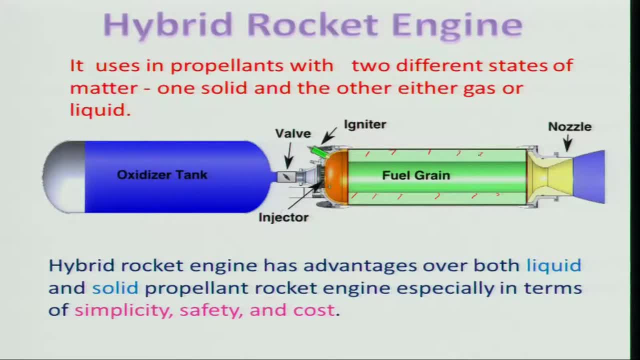 using the fuel. if you look at these are the fuel grain which is being used, solid. this is generally solid and the liquid oxidizer is being used. of course you can think of any other combination, But generally the solid as a fuel. there are several fuel which will be, you know, can be. 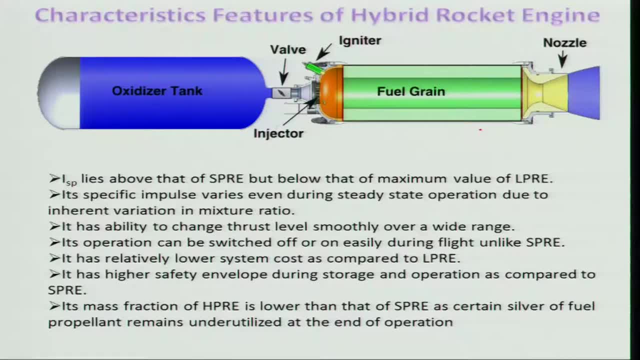 used, But it is having several advantages. for example, it is isp will be lying between the solid propellant rocket engine And with and LPR there is liquid propellant rocket maximum value And it is specific. impulse varies even during steady state operation, of course, due to inner 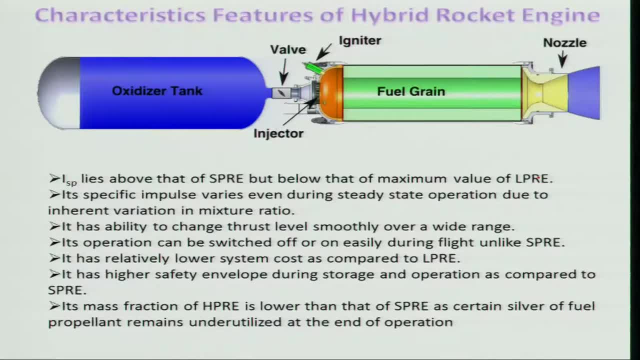 return variation mixture ratio, MR, what we have talked about. It has the ability to change the thrust level smoothly over the wide range. suppose you know you are moving. you want to take a trajectory of path. you can do very easily where the liquid rocket engine one can do, but solid is difficult. 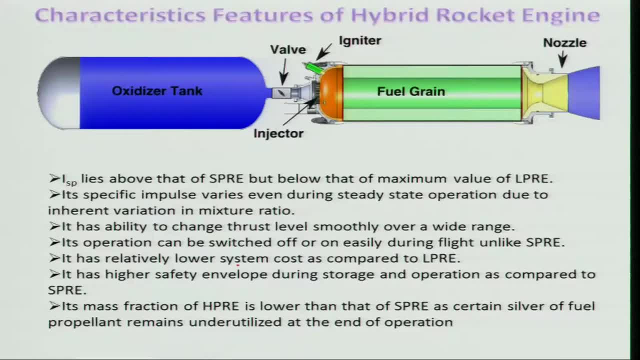 So that is the one advantage. It has: relatively lower cost as compared to LPR, because the system is simple, is only for the one liquid oxidizer, but the fuel line, all the things are there, And it has a higher safety envelope during storage operation as compared to the solid. 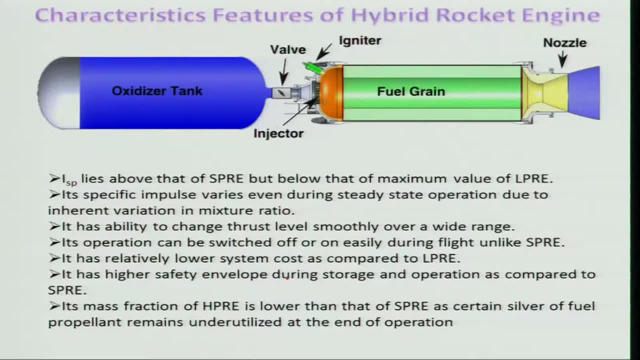 propellant rocket engine because the only fuel- even I you know fuel- is there. nothing will happen unless it comes in contact with oxidizer. So it is also not mixed with the oxidizer, So it is a very safe And it is mass fraction as compared to the solid propellant rocket engine. 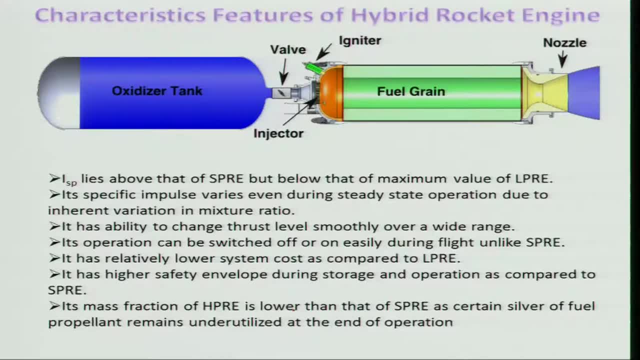 And this mass fraction you know like, is quite lower as compared to the solid propellant rocket engine. And of course the certain silver liner liner means some propellant will be remaining at the end of burner, So that is having higher. So that is the one disadvantage with this. but however, one can design the engines properly. 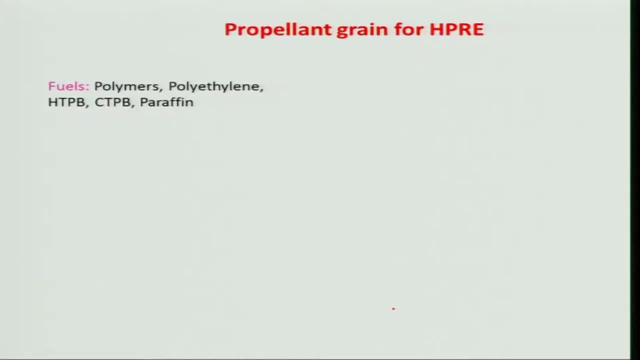 For example, fuels. you can use polymers, polyethylene, STPB, CTPB, paraffin, several other fuels. whatever you use, And oxidizer, you know, like liquid oxygen, what you call hydrogen peroxide, nitrogen tetra oxide, white fuming nitric acid, red fuming nitric acid, several of the liquid. 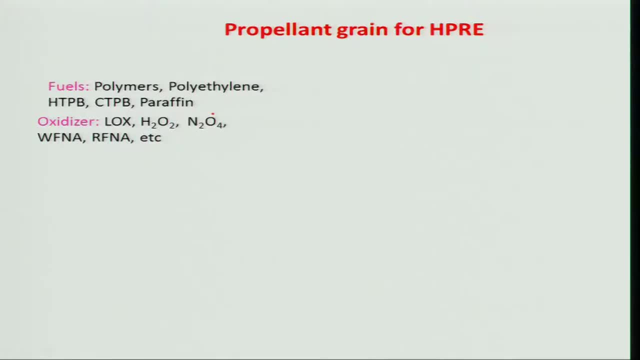 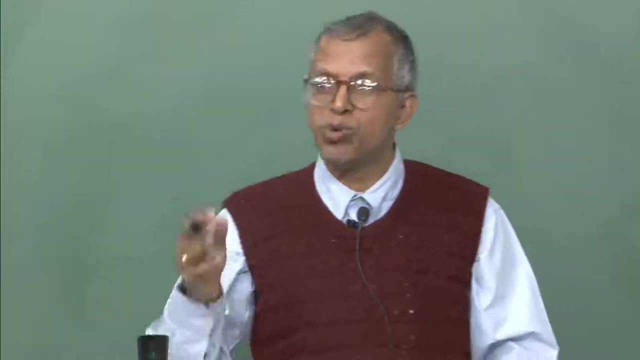 Keep in mind that lot of interest in western countries to have their own, even in the universities of having hybrid rocket, For example, several universities in USA having their own system. students are doing that And in our place only the IIT Madras there. 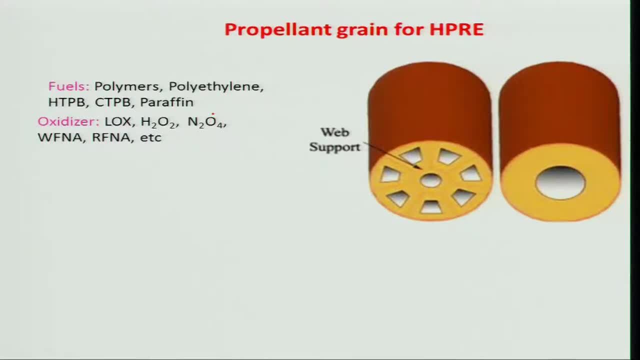 Working on this. if you look at the important one is this is the single port, the grain kind of thing. But the limitation of the this single port is that you know like it will be having restricted surface area, length will be more. Keep in mind that burning rate in case of a hybrid propellant will be order of one third. 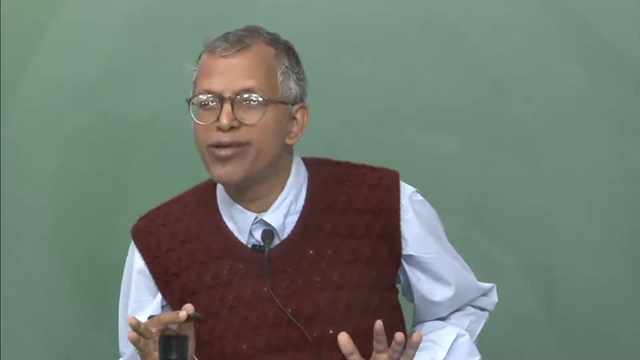 of the solid propellant rocket because in only fuel, So therefore burning rate is reduced. So if you want to have a hybrid rocket, So if you want to have a higher thrust, you will have to go for multiport kind of grain. 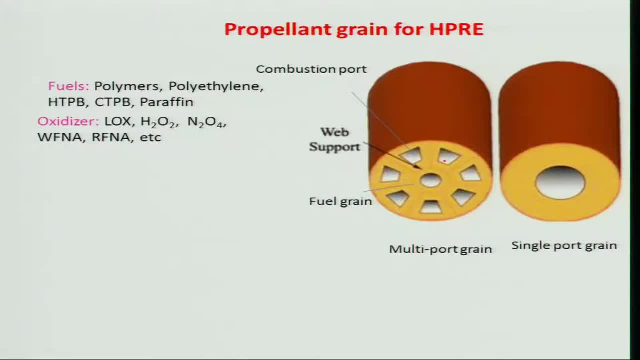 And where the multiport grain design is very important. you know it is not that easy Because if you are having this holes and this having a wave support, it should be supported, otherwise it will fall out out and then it is a very important If you look at if I am having this kind of a port, you know, and if I go on adding this, 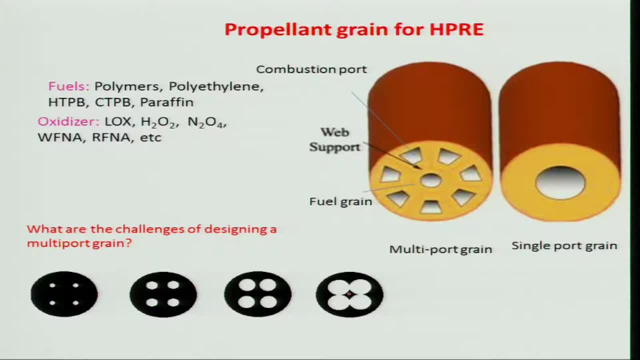 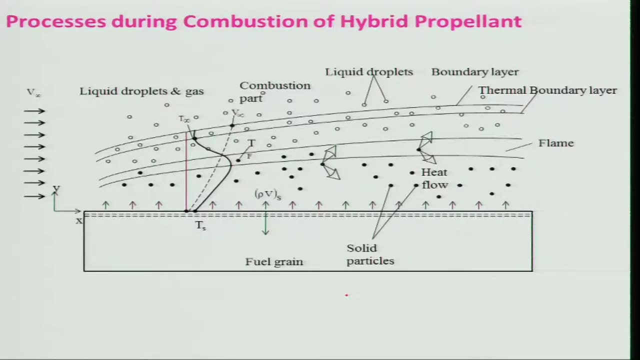 go on receding, There is a place where this portion propellant will fall because there is no nothing supporting. So then, therefore, it will be creating a lot of problem because the thrust will go up or it may explode and other things. So design is very important and let us look at what are the processes involved during 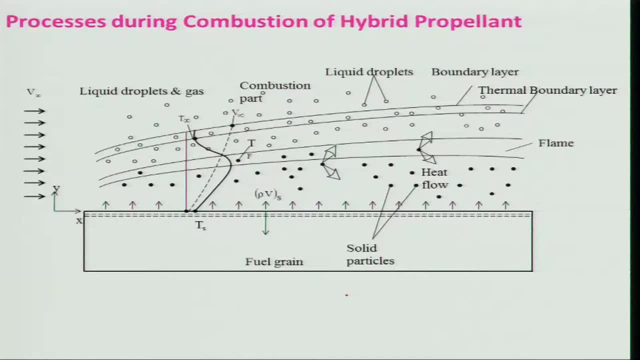 the combustion of hybrid. It is quite difficult, complex, but I will just give a brief overall view. If you look at this, propellant is here solid propellant. these are the liquids. droplets and gases are coming And it will be some heat will be transfer. 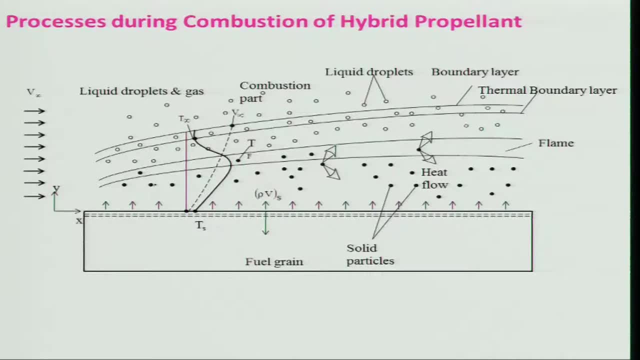 I mean igniting. of course you can do separately, but let us say there is a flame. If it is a flame there will be some solid, you know, some heat will be transferred due to radiation convection because the fluid is moving And this will receded and then this mass will be receding. like you know, it will be coming. 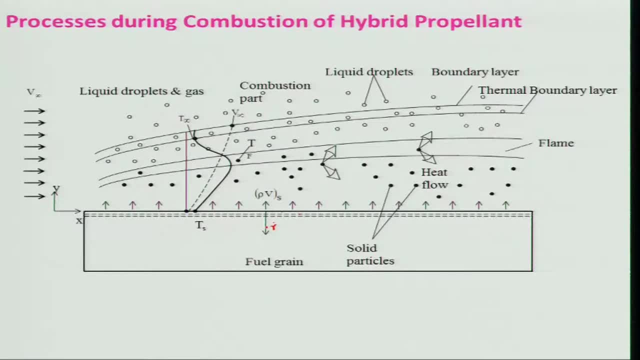 down. it will be regression at a certain you know regression rate And some of the particles also can get into. these are solid particles which will be also passing some heat And then, you know, heat temperature also will be going off and it will be peak at you know. 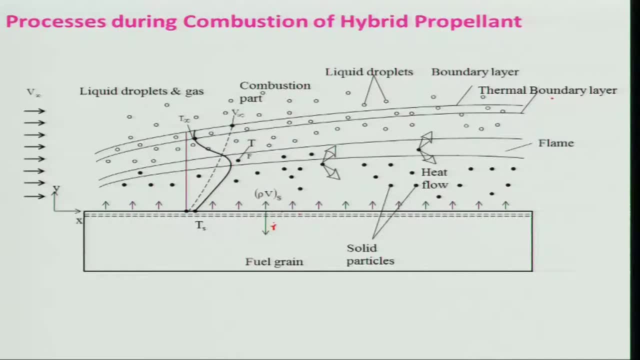 flame temperature here And then it will having. there is a thermal boundary layer, there may be boundary, you know, hydrodynamic or the aerodynamic boundary layer, And then liquid droplets which will be coming, you know, will be vaporizing, entering into. that is a quite a complex process. 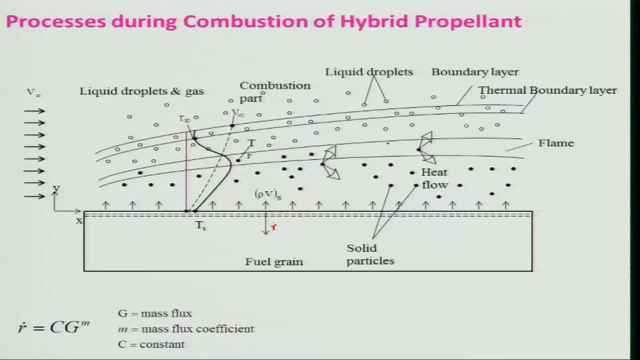 So therefore it is difficult to talk about it, But however one can really model it as a r dot is a, c, g, m, where g is the mass plus is basically rho into v, average velocity. This is the average velocity of mass flow rate which is coming through that and this. 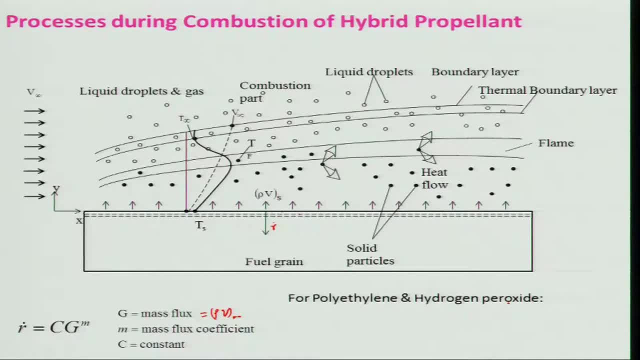 is the constant, And for polyethylene and hydrogen peroxide, if you can get r, dot is equal to 8 g, power to 0.4 mm. centimeter per second if it is a semi-empirical result. So one has to be worry about the unit when you are having. 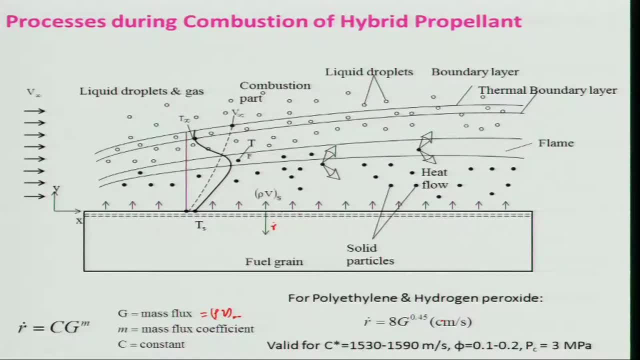 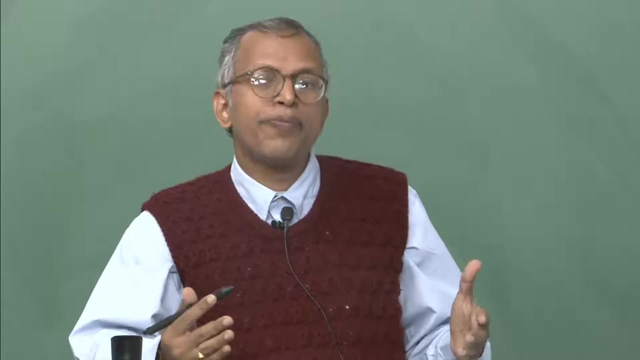 And it can operate over the 1530 to 1590 meter c star. that is the characteristic velocity equivalence ratio: 0.1 to 2, 0.1 to 0.2 and pressure of 3 mega Pascal. So when we are using, you cannot really use that thing for all, like your solid problem.